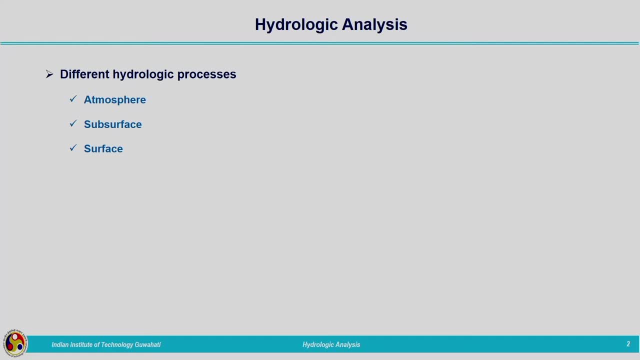 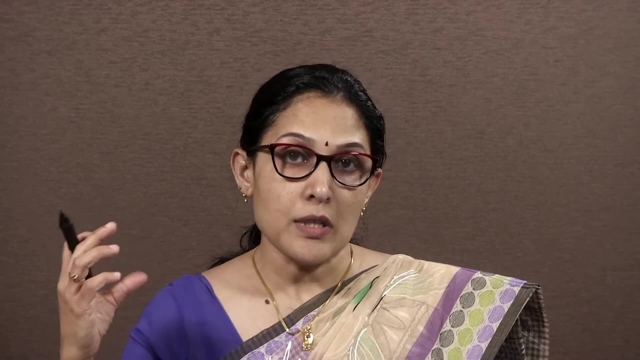 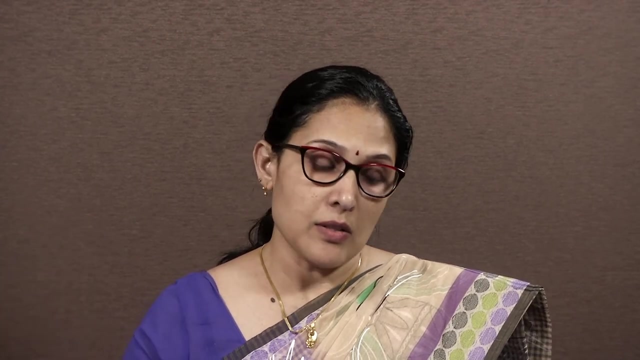 way. atmospheric water, subsurface water and surface water. we have covered. Now we need to make use of these processes for understanding the impact of these things. So we are going understanding their impact on the catchment or watershed or any hydrologic system. so in this, 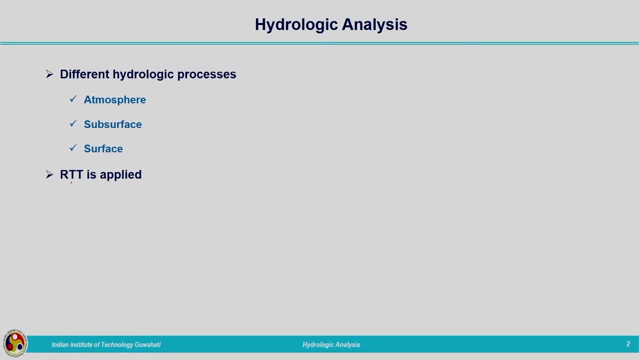 what we have done. we have made use of RTT for understanding different processes and we have derived physical laws related to different processes. and in the control volume approach we were not giving much emphasis to internal dynamics of flow. actually, it is not required. the internal dynamics of the flow is not required in the control volume approach. what is important? 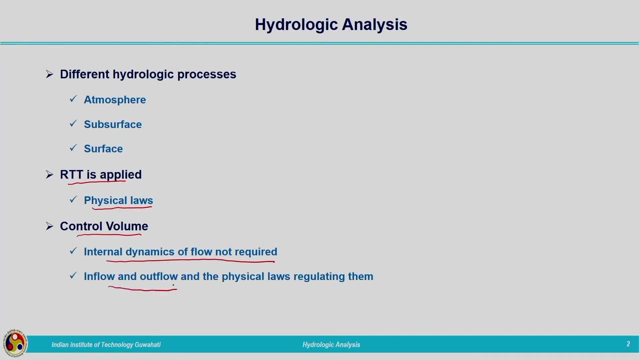 is that the inflow and outflow and the physical laws regulating them, different physical laws. we have seen conservation of mass, conservation of momentum and conservation of energy, depending on the process which was decided in the control volume approach. so various factors such as energy we are dealing with. we were making use of different fundamental laws. So here, by making use of RTT, 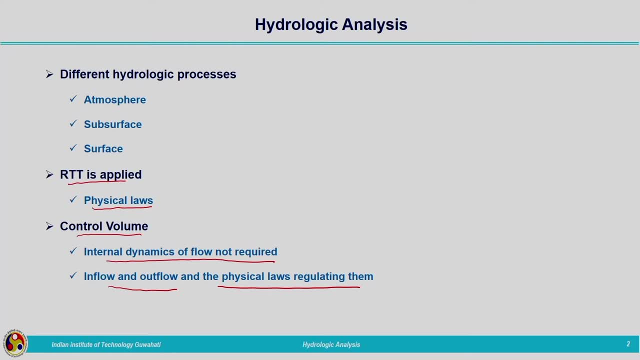 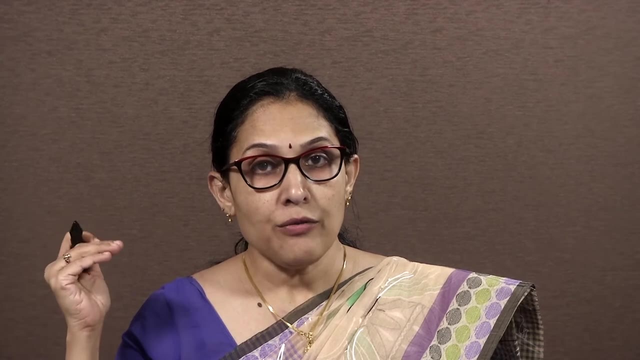 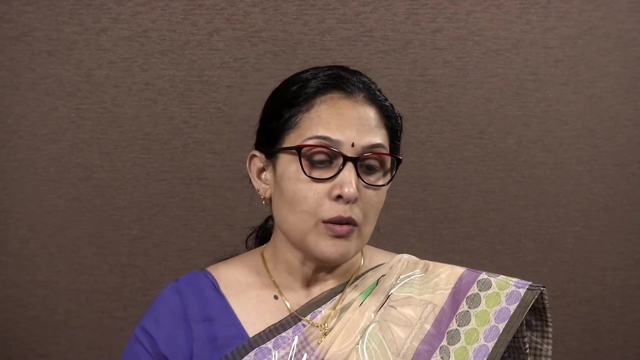 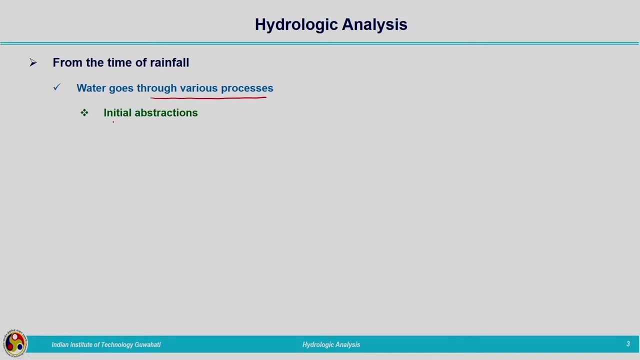 what is important is that the inflow and the corresponding outflow and the fundamental law which is governing that particular process. So we have studied, whenever there is a rainfall or storm is occurring, what are the different processes taking place before it reaches at the outlet as runoff. So from the time of rainfall, water goes through various processes such as: 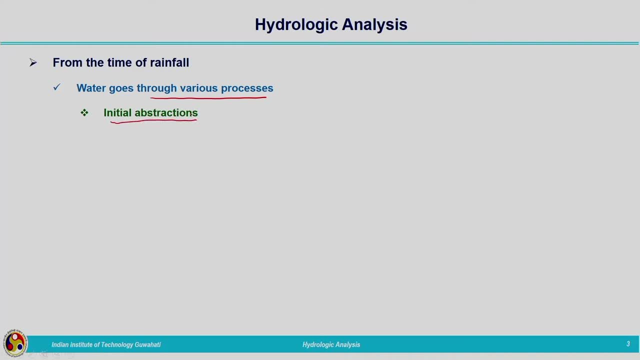 some amount of water is lost as initial abstractions, then some amount will be infiltrating into the ground and after that only it gets converted into the surface and substrate So directly, whenever a rainfall is occurring, it will not be directly converted to runoff. There are cases in which direct conversion taking place, in which entire area is impermeable. 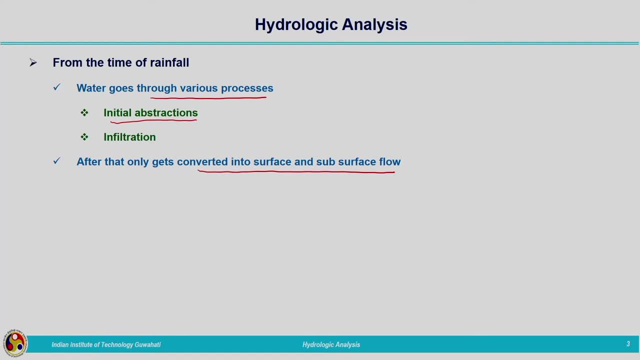 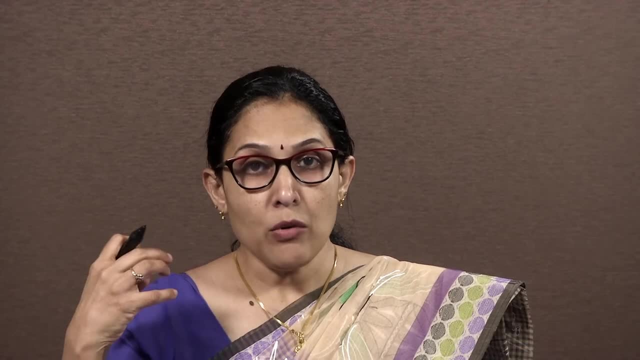 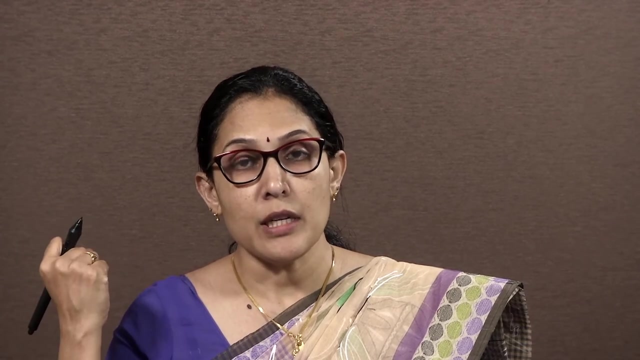 So whatever rainfall is occurring, that will be translated to runoff. but in general way, whenever a rainfall is occurring, some amount of water will be lost as initial abstractions, and part of the water will be converted to runoff. So we have studied this in a very. the rainfall will be infiltrating into the ground and remaining after satisfying all the storage. 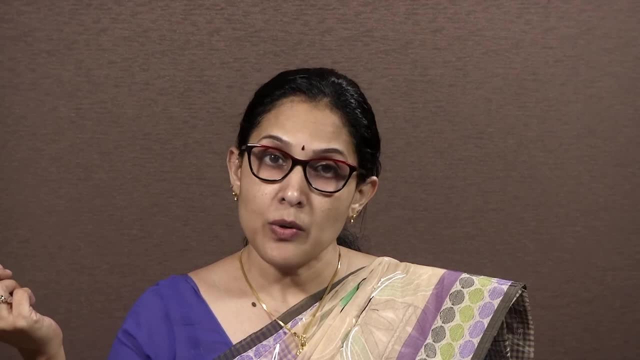 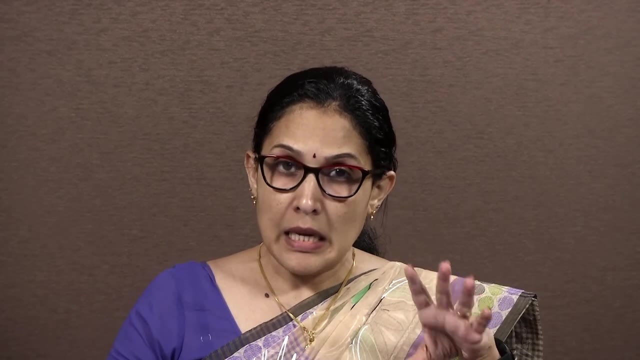 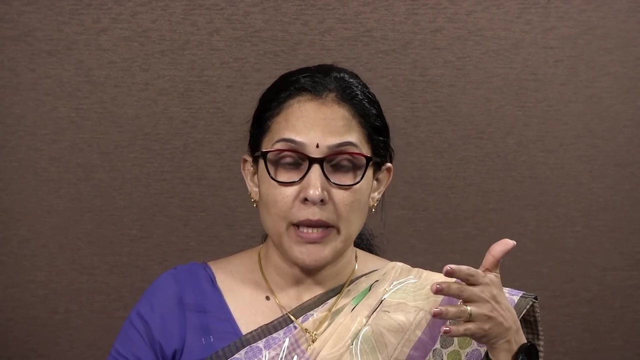 components remaining, one only will be contributing towards the surface and subsurface flow, So before it is reaching at the outlet of a watershed as a runoff or interflow or base flow. so so many processes will be taking place. So the process of translation of rainfall into runoff is 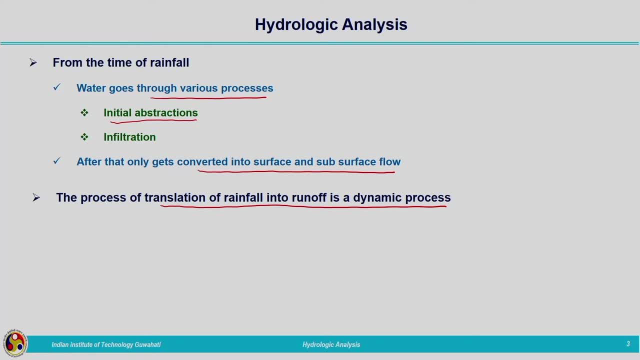 a dynamic process because satisfying this storage, we have studied different types of storages present on the surface of the earth and beneath the surface of the earth. So once the storage components are satisfied, then only the runoff or the overland flow is starting. that is very complex. 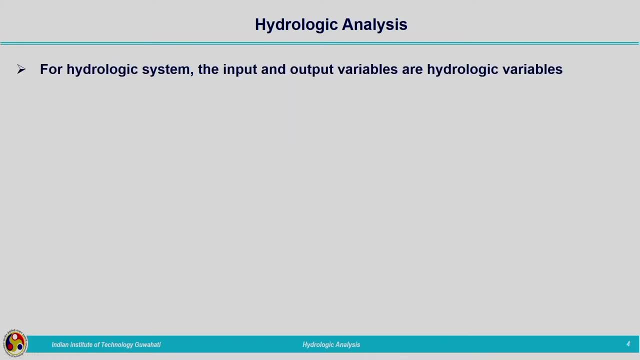 and also non-linear. For understanding hydrologic analysis, first we will look into a hydrologic system. So hydrologic system is the one in which the input and output variables are hydrologic variables. So we have studied what is meant by a system. It is acted upon by an input and based on the 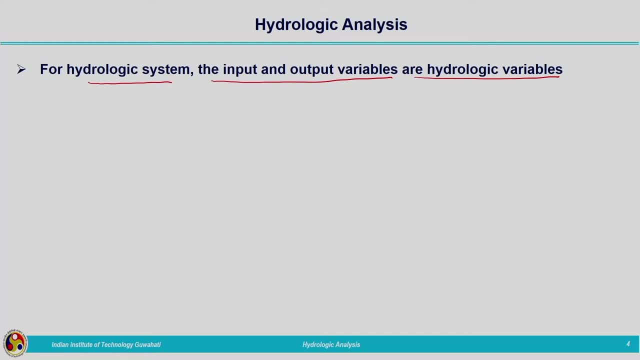 processes which are taking place within the system, we will be getting some output. In the case of a hydrologic system, the inputs and outputs will be of hydrologic variables. We can consider the example of a catchment. Catchment can be considered as a system, So the catchment is. 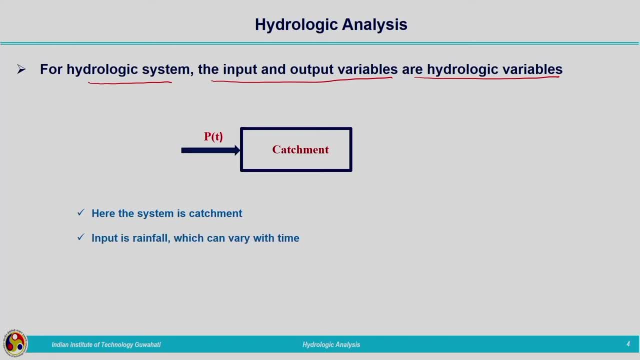 acted upon by an input, pt, For example, that input can be considered as rainfall. This rainfall is varying with respect to time and also with respect to space, So the rainfall is represented by means of a hydrograph that we have already studied while explaining atmospheric water. So this 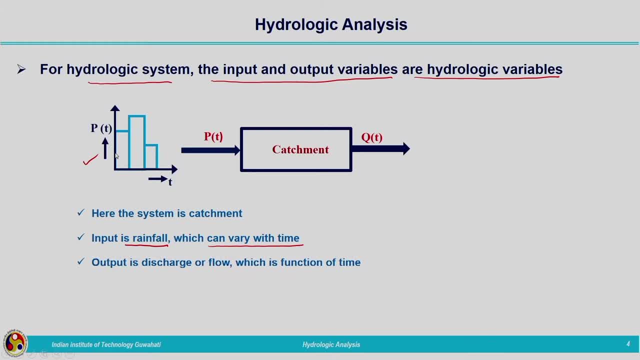 rainfall is falling on the catchment and output is produced, that is the discharge or outflow. This is also a function of time, So that can be represented by means of a hydrograph. So the time distribution of the flow at the outlet of the catchment- we have seen it- can be represented by: 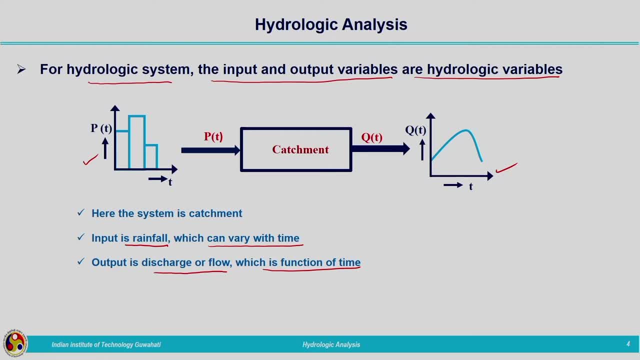 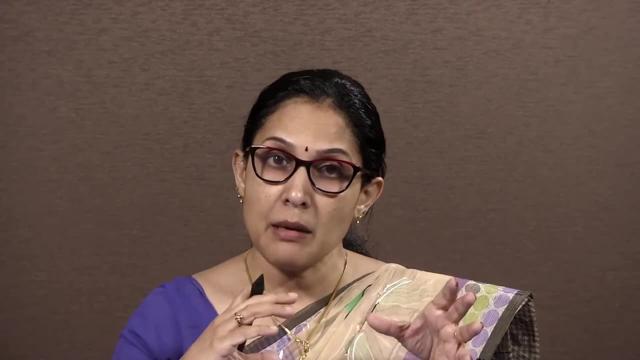 means of a storm hydrograph. So rainfall is falling on the catchment and, after certain processes taking place, the remaining water will be converted to the runoff. this is the complete hydrologic system. system is acted upon by means of certain hydrologic input and certain output. 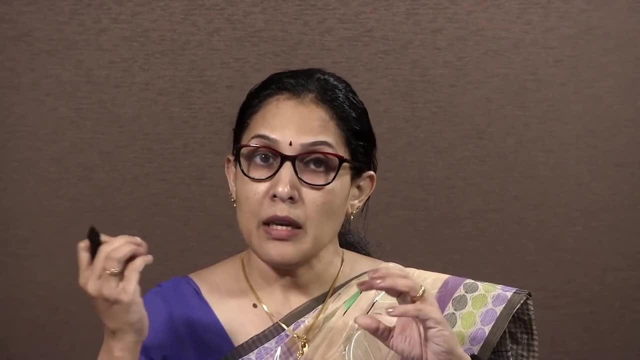 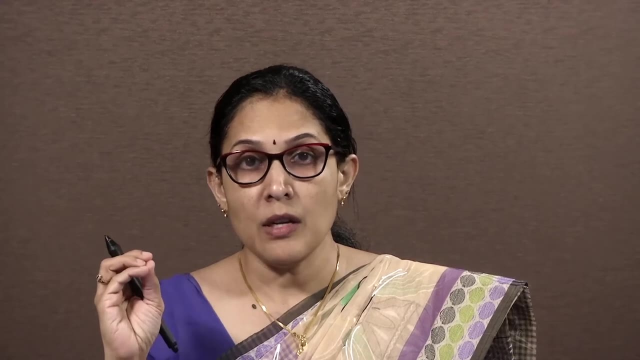 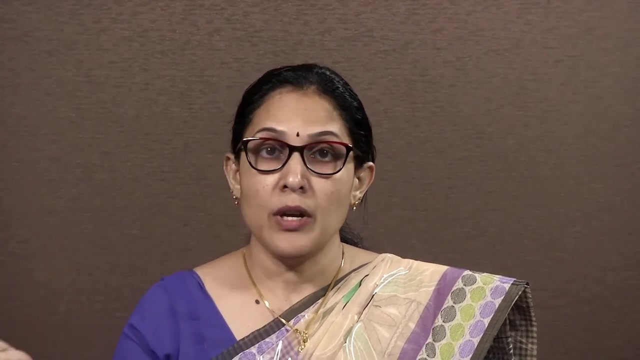 is produced. that is also hydrologic variable. in the case of rainfall, it is the runoff. so here we need to understand different processes thoroughly, which we have already discussed in previous modules, and how this rainfall is translated into runoff. that is what we are going to study in this. 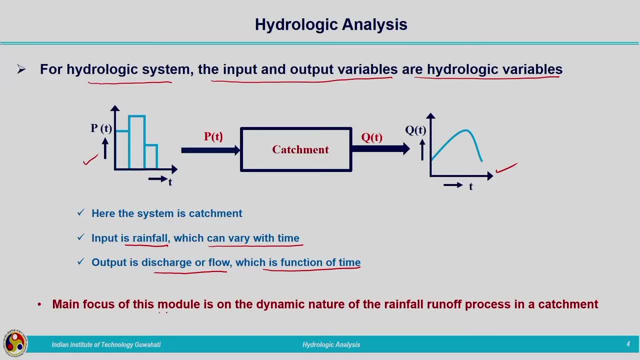 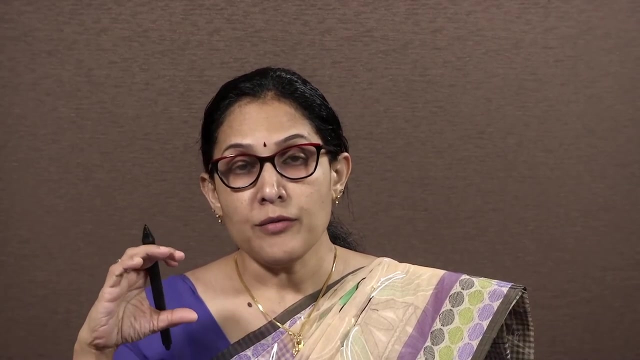 module. so the main focus of this module is on the dynamic nature of the rainfall runoff process. in a catchment, rainfall runoff process means we are having some rainfall which is acting on the catchment. after different hydrologic processes it is converted into runoff. so when, Whenever a rainfall is occurring after satisfying the storages, we will be getting the runoff. 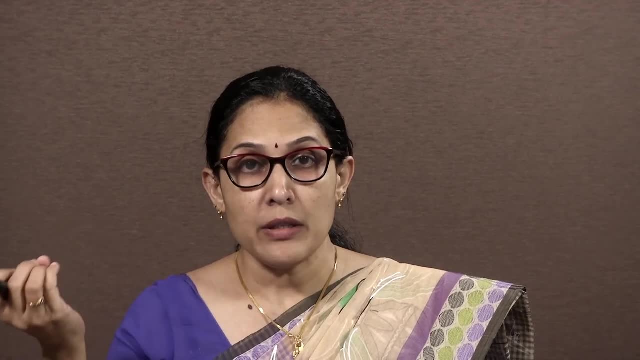 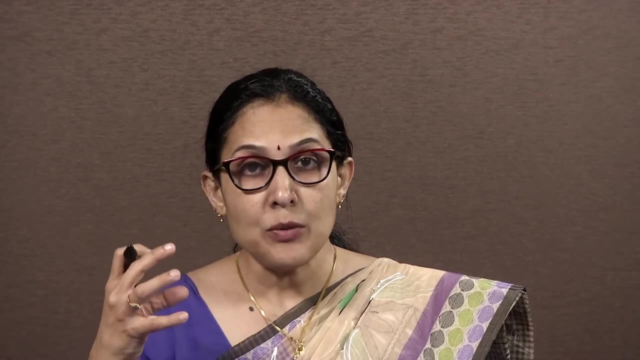 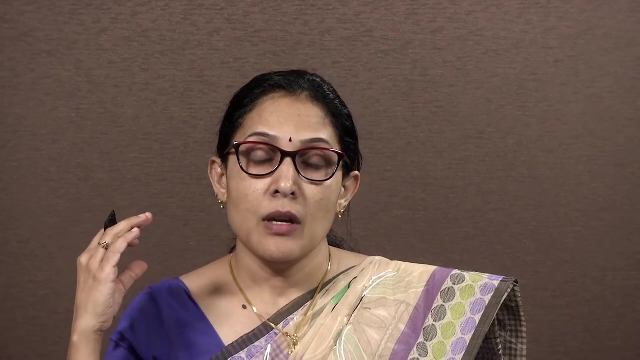 So if we want to calculate the runoff at the outlet of the catchment, we need to have understanding about the inflow and also the catchment properties. For example, if we are having a catchment which is having different storage components, different ponds are there, lakes are there, channels are there? 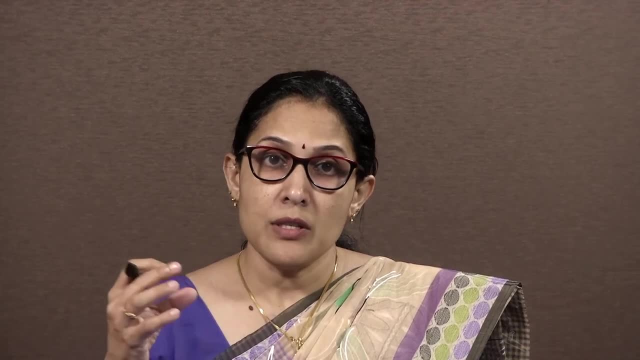 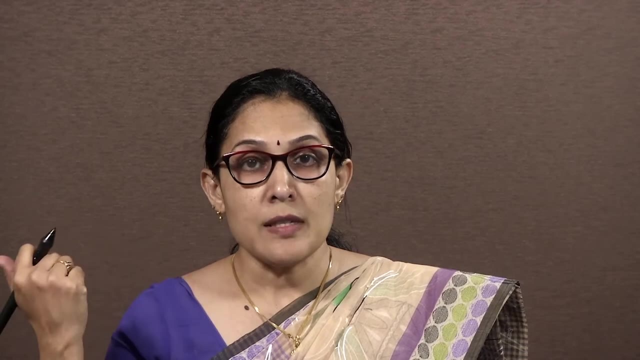 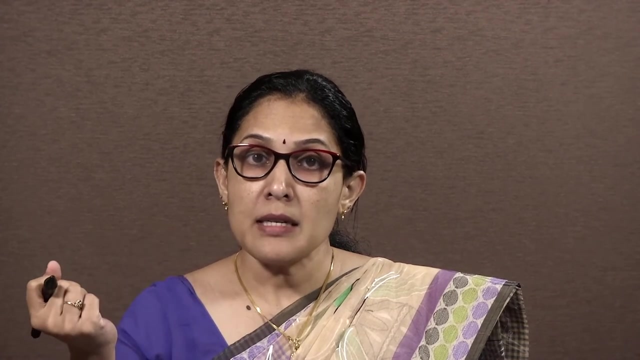 And there is a catchment in which there is no features like this. So same amount of rainfall is occurring in both the catchments. The flow which is experienced at the outlet of the catchment will be different, So we need to have proper understanding of different hydrological features present in a catchment. 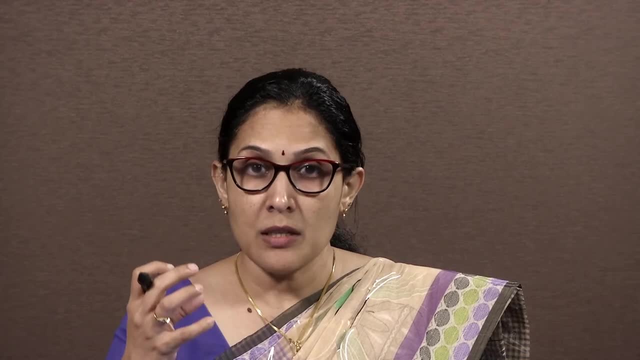 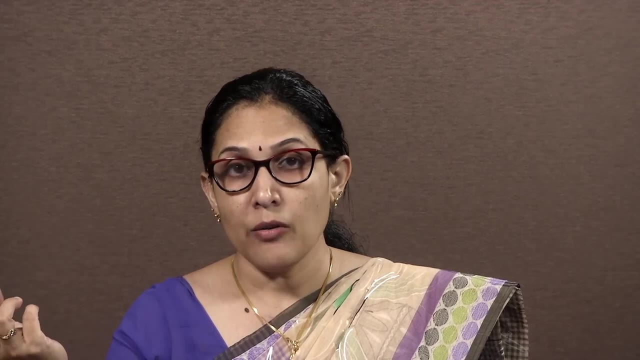 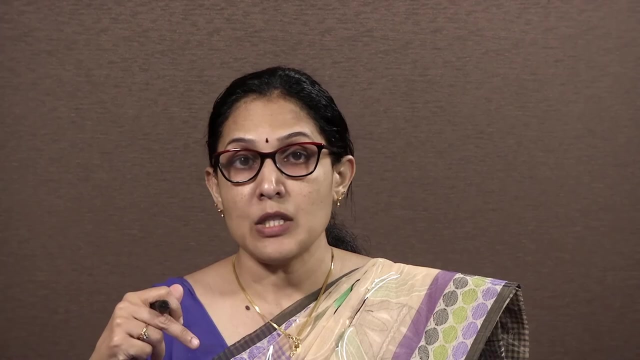 And also what is the type of inflow experienced by the catchment. So, based on these two, only we can We can predict the runoff, We can calculate the runoff. So this rainfall runoff process purely depends on the processes which are taking place in the catchment. 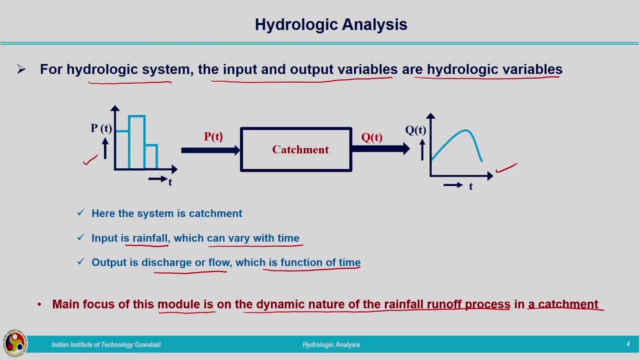 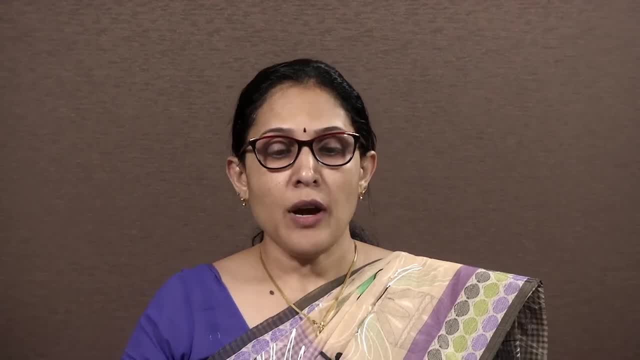 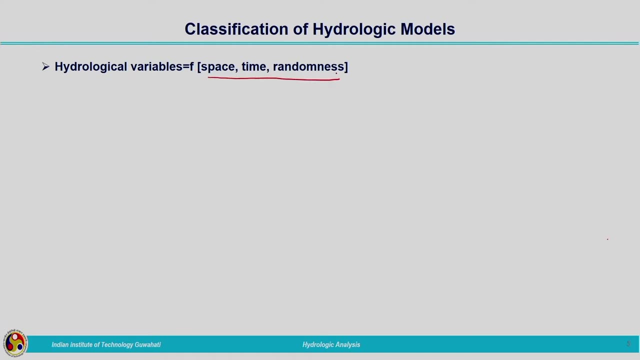 This dynamic nature of the rainfall runoff process can be studied by means of different models. So let us first see the classification of hydrologic models. Hydrologic variables can be functions of space, time and randomness, So this randomness is a new terminology as far as you are concerned. 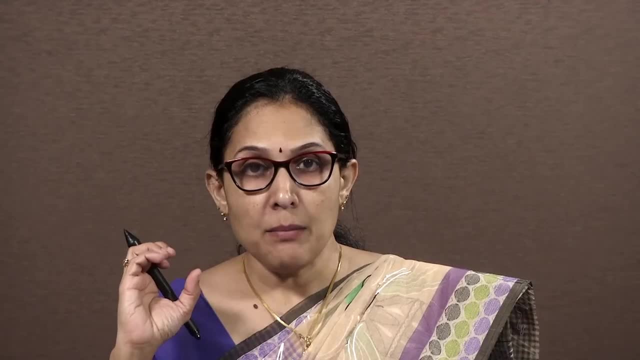 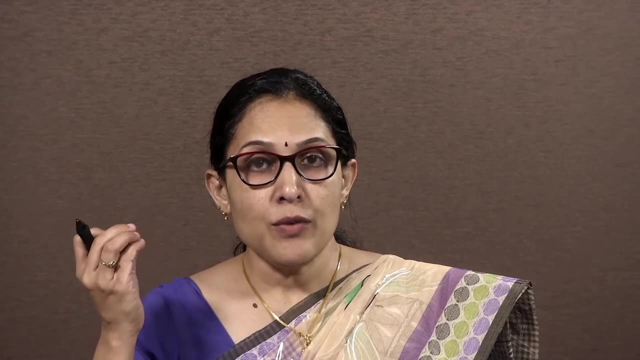 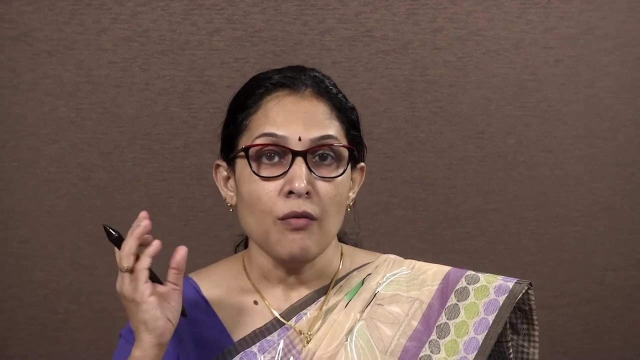 What is meant by this randomness When we are discussing about certain hydrologic variable? For example, if you are considering rainfall, Rainfall which we are experiencing today will not be the same as the one which we have experienced one day before. It cannot take a fixed value at a particular point for varying. 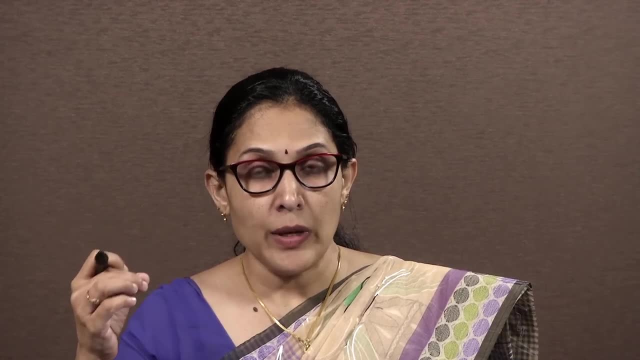 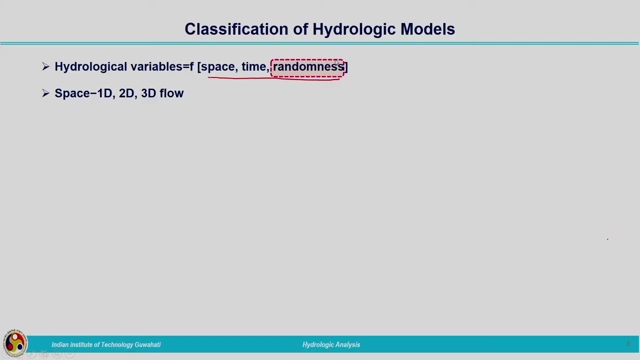 Time. So in a catchment at a particular location we cannot forecast that the rainfall will be exactly of this much amount, And when we talk about space, it can be 1D, 2D or 3D. That is, one dimensional, two dimensional or three dimensional. 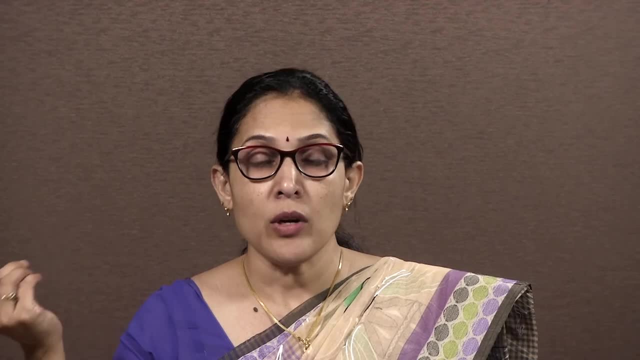 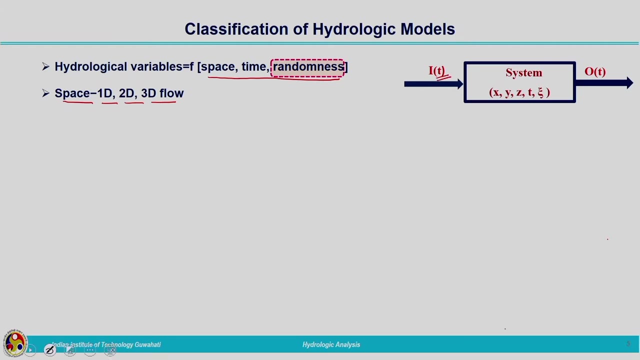 For certain types of studies, one dimensional models will be giving sufficient answers. Now, when we are considering the system, it is acted upon by an input And it produces output, So system can be represented as a function of x, y, z, t and zeta. 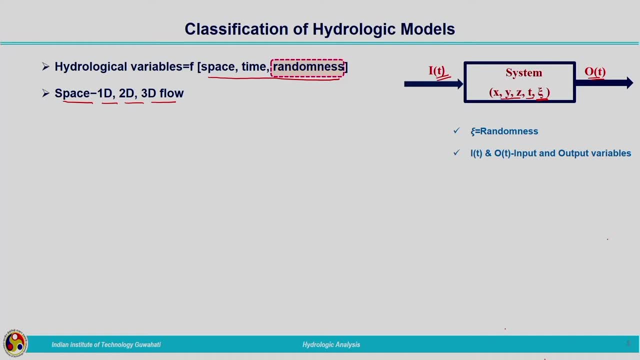 x, y, z is representing all the three dimensions in space And t is the time, And zeta is representing the randomness involved with the hydrologic variables. It and ot are the input and output variables. For example, input can be rainfall. 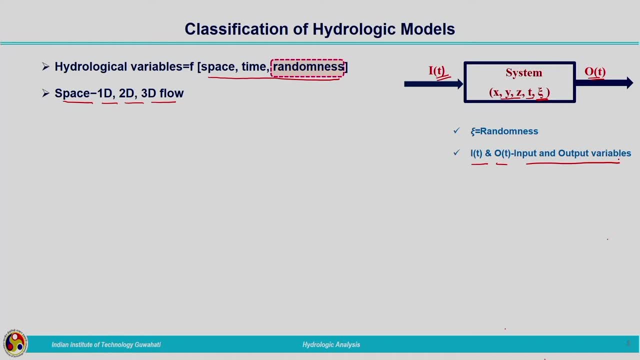 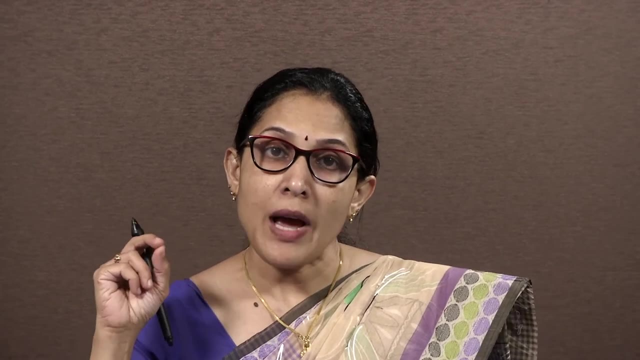 And the corresponding Output from the catchment can be outflow or runoff, So these two can be considered as consisting of certain amount of randomness. For example, if we are talking about rainfall, we cannot expect the same value, a fixed value of rainfall at a particular point in space for all the times. 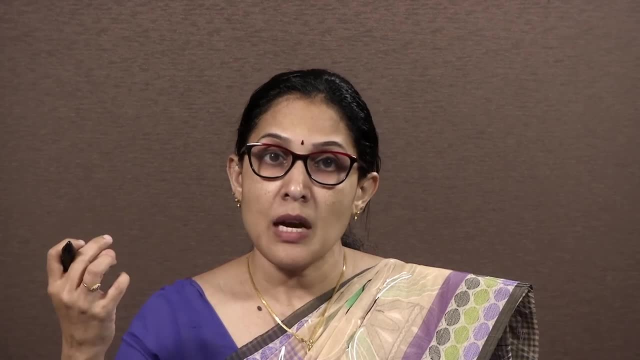 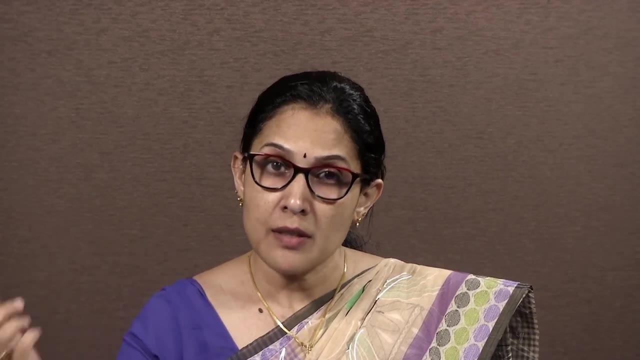 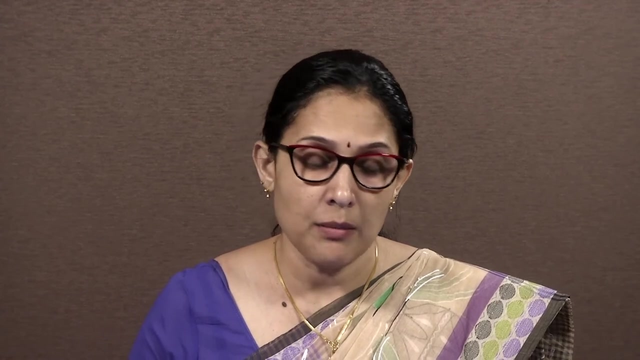 There are certain uncertainties involved with these type of hydrologic variables, So that also need to be considered, So that also need to be taken into account while modeling such kind of systems. That is why we are incorporating randomness involved with these hydrologic variables. 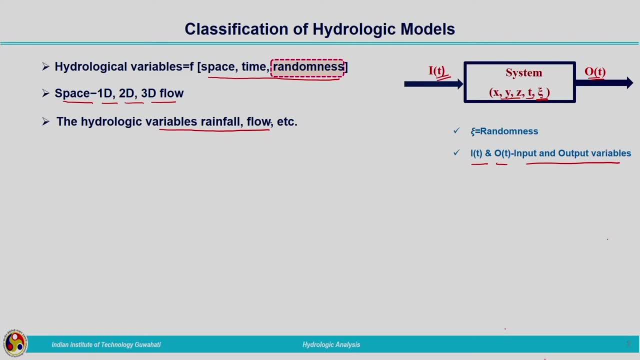 So hydrologic variables such as rainfall, stream flow, etc. These variables vary from one place to another, It varies with respect to time And some amount of randomness is involved with these variables. So this is the randomness, Randomness. 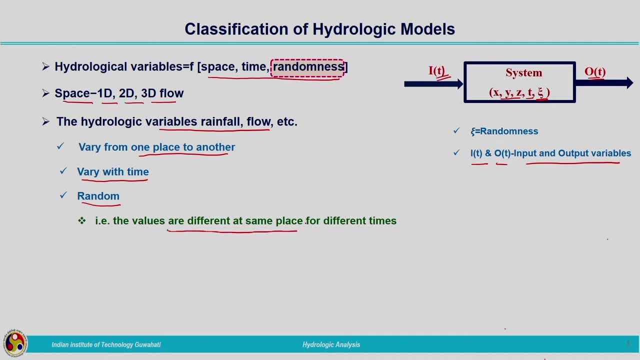 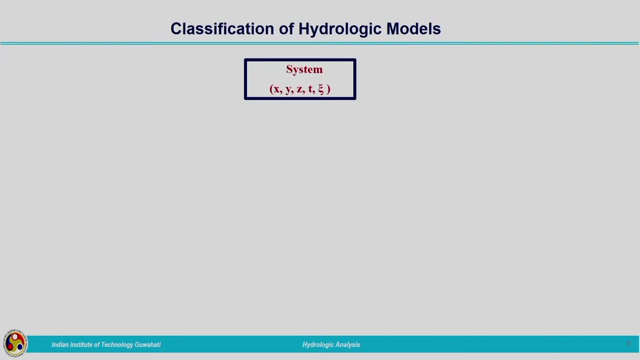 In the sense the values are different at same place for different times. We cannot expect a fixed value of rainfall at a particular place for all the times Because of the uncertainties involved with the water vapor dynamics. Now coming to the classification of model. 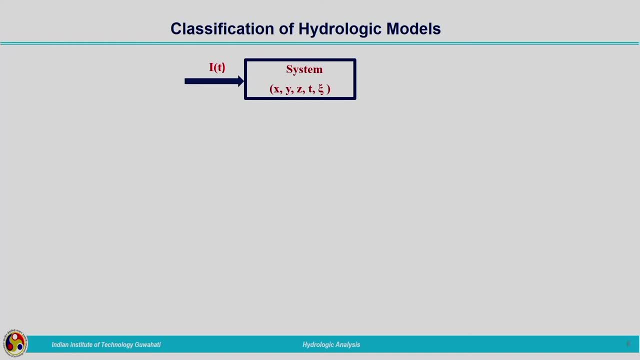 I have already shown this flowchart in the previous slide. System is acted upon by input IT and output OT. We can see different types When we consider different dimensions: x, y, z, three spatial dimensions, temporal dimensions and randomness is also incorporated as a dimension. 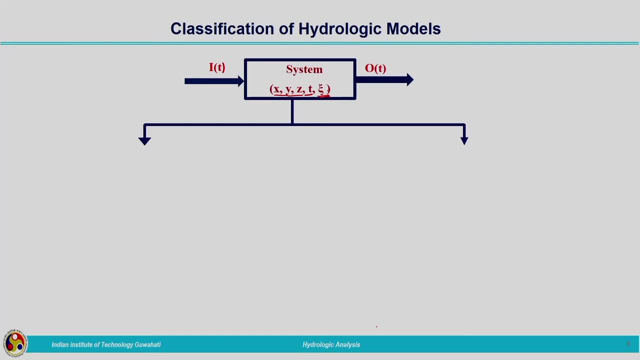 So by incorporating all these five, we can divide hydrologic models into deterministic models and stochastic models. What is meant by deterministic model? Very simple deterministic model can be explained by means of an equation. Very simple deterministic model can be explained by means of an equation. 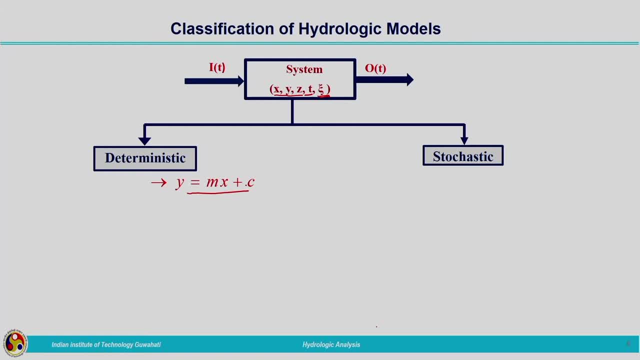 Very simple deterministic model can be explained by means of an equation: y is equal to mx plus c. Everybody knows y is equal to mx plus c is representing a straight line in x- y plane. So that can be considered as a deterministic model. 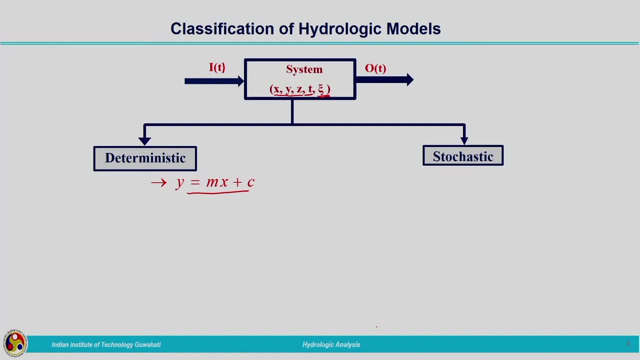 Simple model, And when we talk about stochastic model, it can be represented by an equation. In addition to this, y is equal to mx plus c. we are having a randomness component, zeta. So you look at these two Equations: y is equal to mx plus c and y is equal to mx plus c plus zeta in the case of a deterministic model. 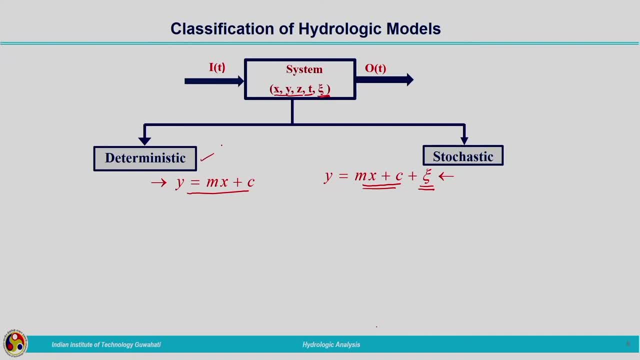 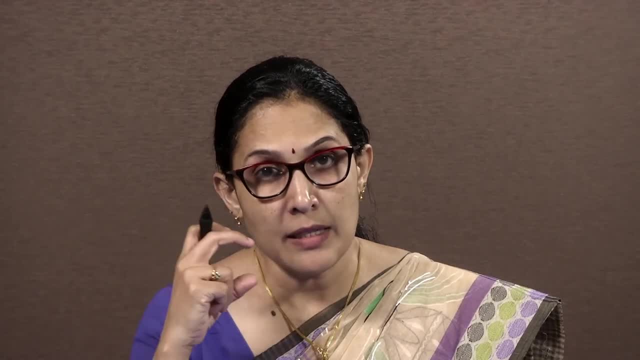 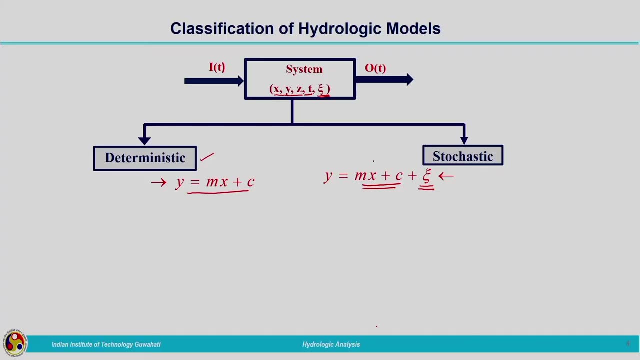 for one value of Vx, We will get balloon value for Y corresponding to single value of input x. we'll be getting single output Y. But in the case of stochastic model, even though X is represented by means of a single variable, we are: 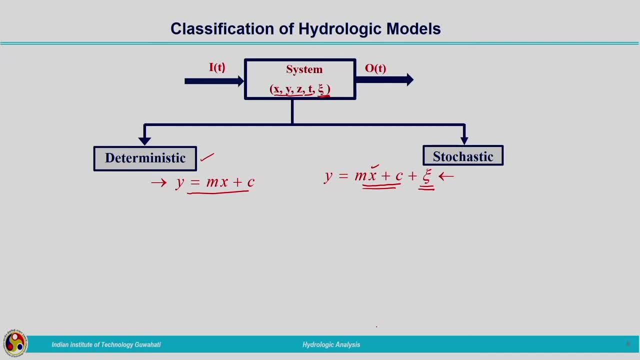 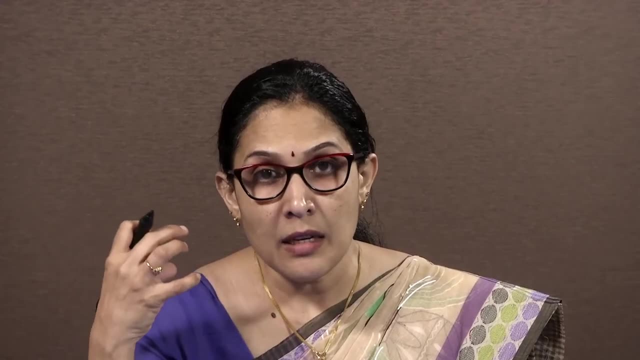 having a randomness component zeta. So for a single value of x there can be so many outputs depending upon the component zeta. So that way, incorporating that randomness is a complicated process that is incorporated in the case of stochastic models. So this is a simple example. 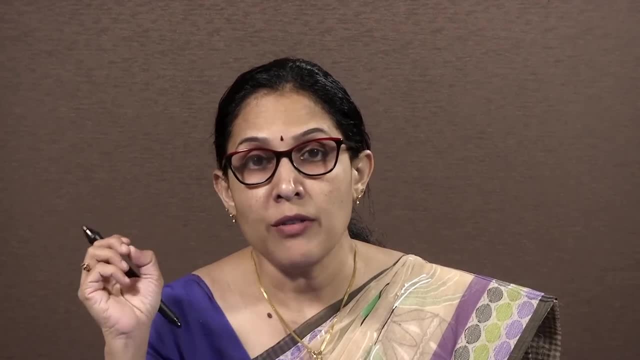 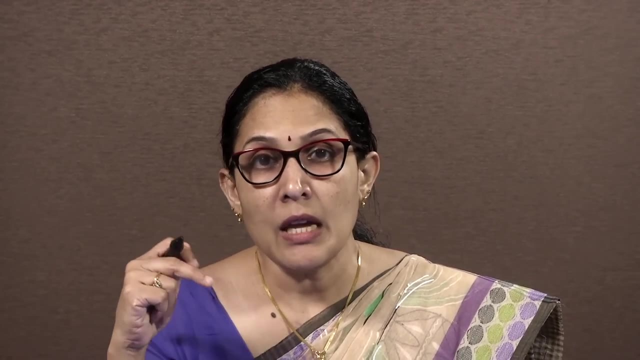 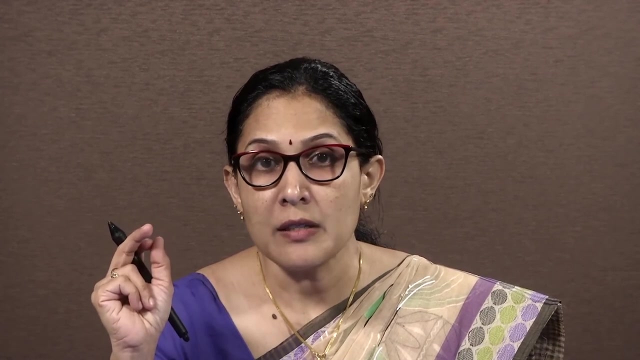 I have taken y equal to mx plus c. for every x you will get a single y value that can be plotted as a straight line. But in the same way, if the randomness is incorporated in that particular equation for a single value of x or because of the uncertainty of randomness related to x, 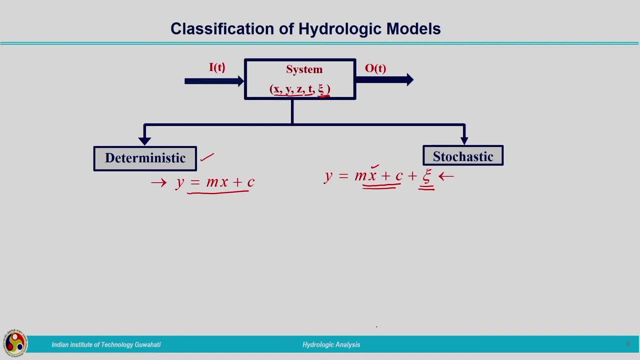 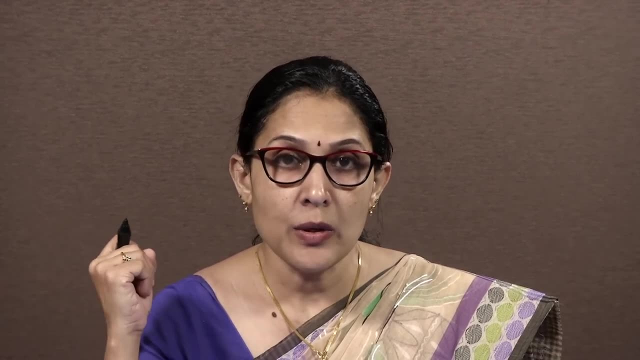 there may be different values corresponding to y. It will not be a fixed value. So that is the fundamental example I have taken Difference between the deterministic model and the stochastic model In detail you will study when you study the course on stochastic hydrology. So here I am not going deep into that particular. 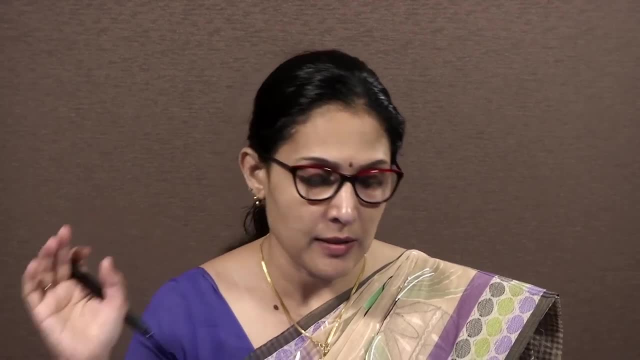 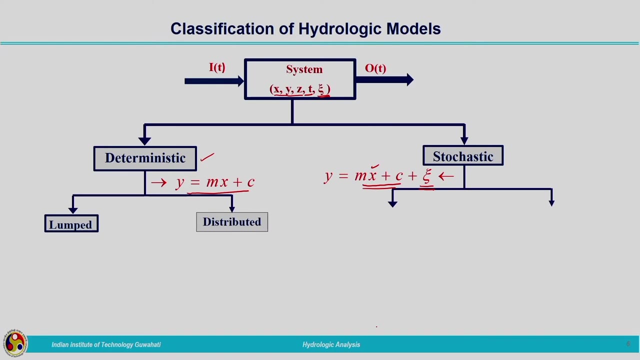 topic. We will be discussing only deterministic models And again, deterministic models can be classified into lumped model and distributed model. What is the difference between lumped and distributed? Lumped model is the one in which space variation is the one in which space variation. 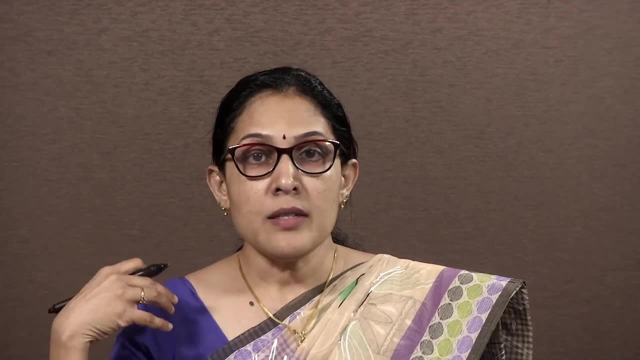 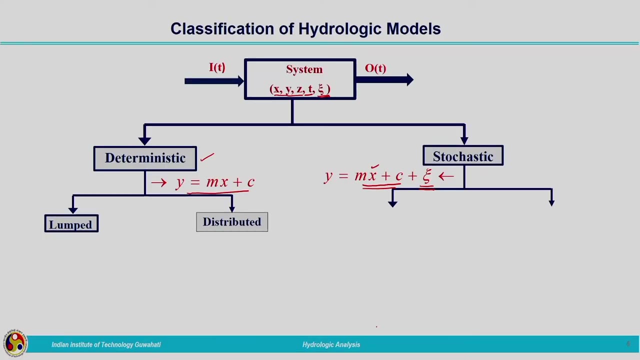 is not taken into consideration, And distributed one is the one in which space consideration is taken care. So lumped model again can be divided into steady, unsteady, and distributed model also can be divided into steady and unsteady models. So what is meant by steady and unsteady models? 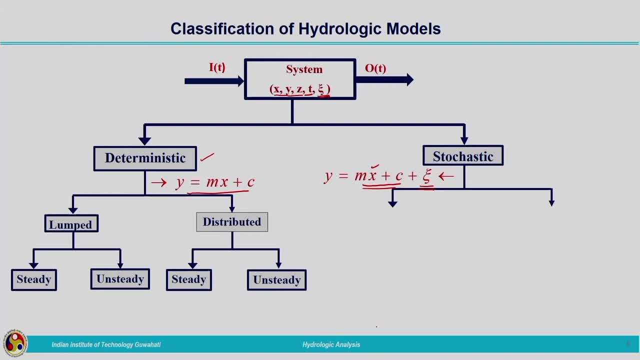 you know already, Steady model is the one in which variation with respect to time is not taken into account. On the other hand, in the case of unsteady models, the variation with respect to time is taken into account. So both lumped and distributed models can be divided into steady. 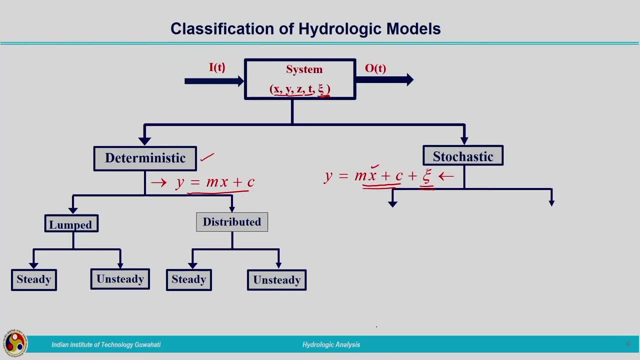 and unsteady models. So lumped model is the one in which space variation or the variability with respect to space is not taken into account, But that is also incorporated in the case of a distributed model. Now, while coming to stochastic, Stochastic model that also can be divided into two, That is, space independent and space correlated. 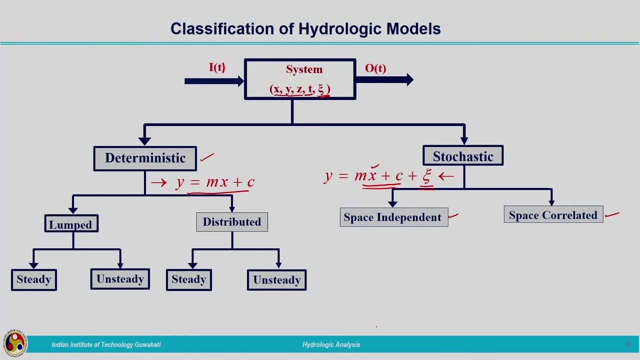 As in the case of deterministic model, we have divided into two. That is lumped and distributed. Here, in the case of stochastic model also, it is divided into two, But we are not calling it as lumped and distributed. We are considering it as space independent and space correlated. 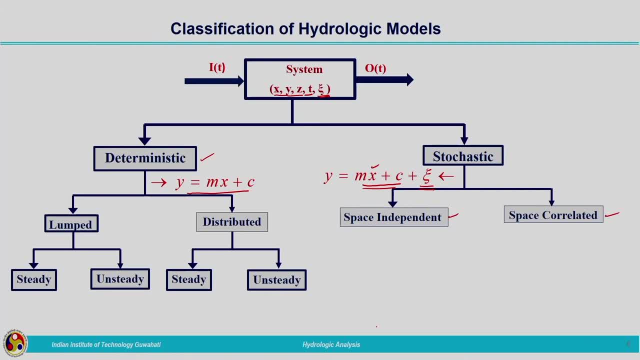 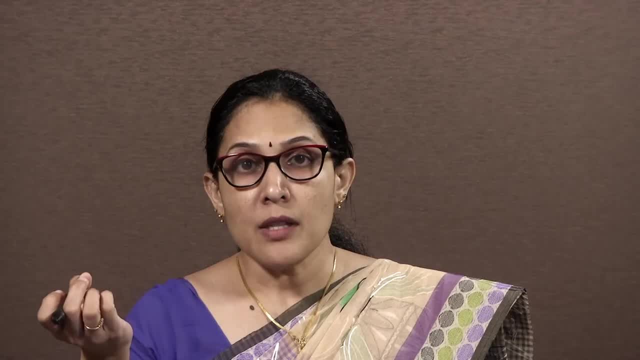 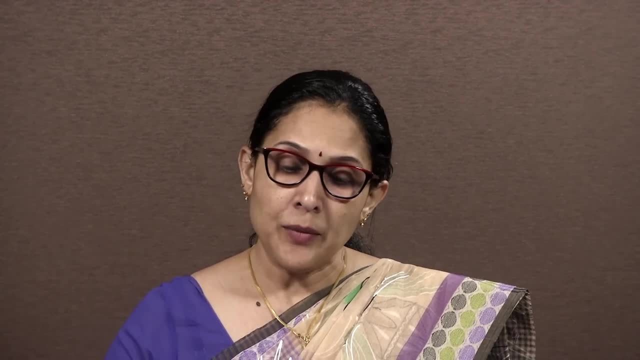 That is, lumped model is the one in which, independent of space, The same thing is known as space independent model under stochastic consideration And in which the variation with respect to space is incorporated. That is termed as space correlated stochastic model, And here also the classification with respect to time is there. That is time. 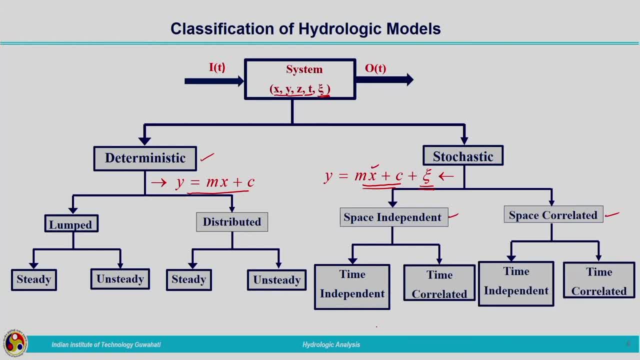 independent one and time correlated. In both the cases, time independent and time correlated models are there. That is, one is depending on the time and the other one is independent of time. That is, in the time independent model the variation with respect to time is not taken. 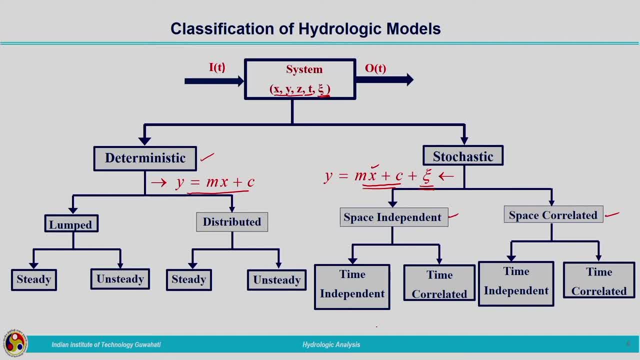 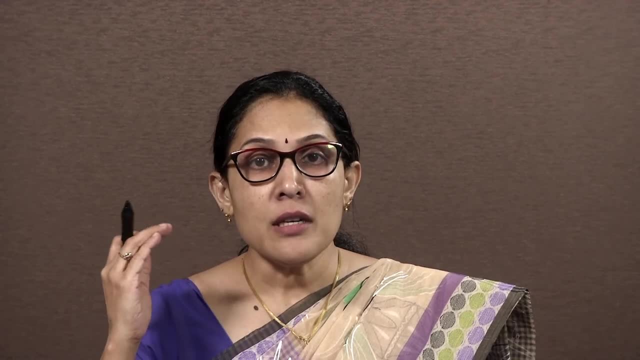 into account. Time correlated one. the variation with respect to time is taken into account. So here in this module we will be mainly discussing on lumped unsteady models. Space variation is not taken into account. The variation with respect to time is taken into account. 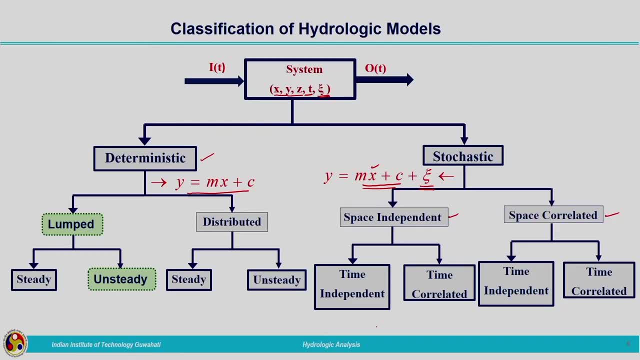 So generally that model is called as lumped model. The general classification of hydrologic models we have seen with the help of this flowchart, That is main classification, is deterministic and stochastic. We are going to look into deterministic model only. Deterministic itself can be divided into lumped and distributed. 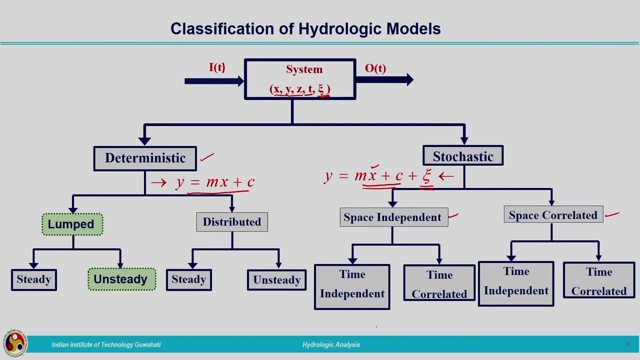 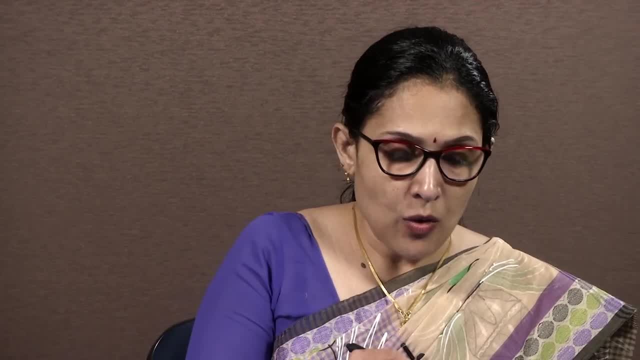 And under lumped, steady, unsteady. out of that we will be looking into unsteady, lumped model in this module. So hydrologic system, when we talk about it, deals with the range. So we are going to look into the range of unsteady, unsteady, unsteady model in this module. So 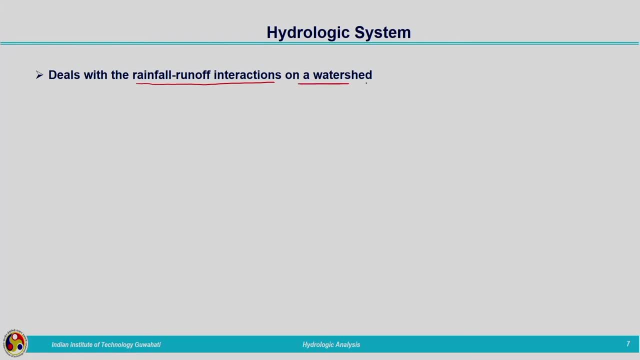 hydrologic system. when we talk about it deals with the range of unsteady, unsteady, unsteady. So in this module we have seen that, of course, why it is called as grypserry best unsteady one, Because none of the standard methods which we generally succeed in working out actually 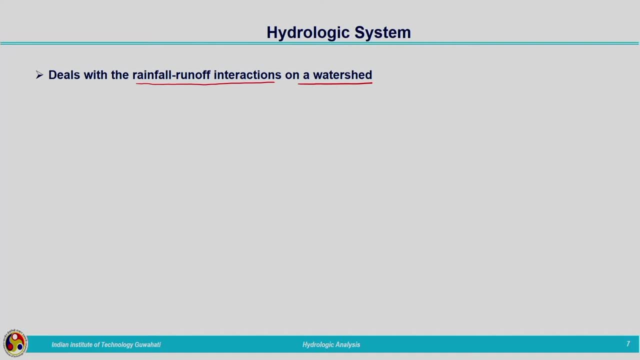 work independently or well with Dr rekode. This is exemplified work in our worries or questions. So with interpretation of the applicant we can have the point that the assumptions in our algorithm as presented in the newsletter are quite accurate. So we can say that we can deliciously cheddar a conceive person with, now, these arguments. 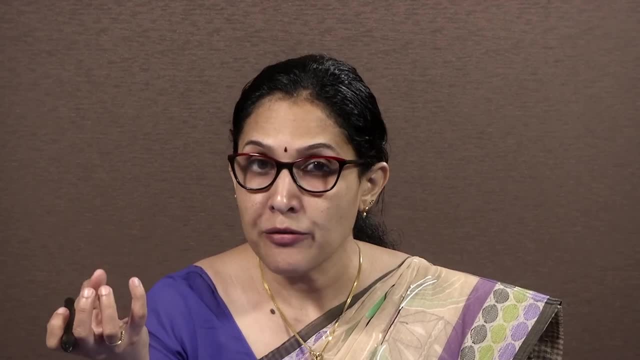 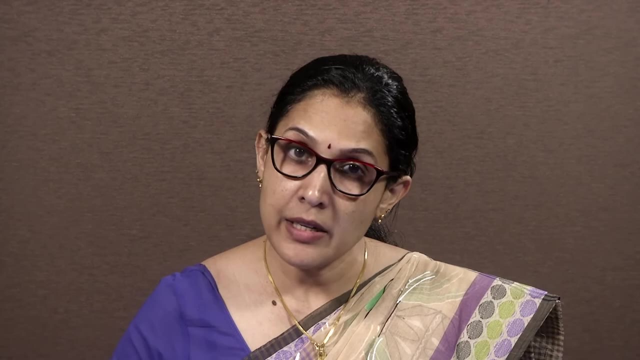 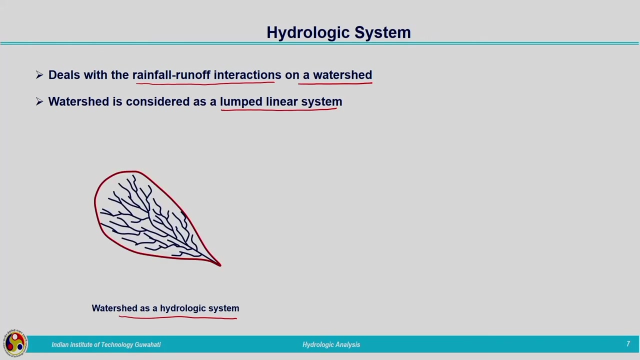 and their objections, which usually can be interpreted. it Thisition S, K, S to different storage components, or we are considering all these relationship in the linear way. now we can look into a watershed as a hydrologic system schematically. so this is a watershed. what is meant by a watershed? you know already. this red line is representing the watershed. 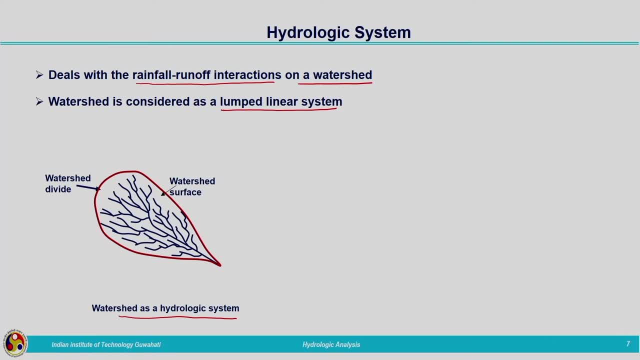 divide line and we are having the watershed surface- and if you are considering the watershed as a system, this can be considered as the system boundary- and the watershed is experiencing a precipitation, represented by it, and we are experiencing an outflow at the outlet, which is represented by the stream flow qt. this is the schematic representation of hydrologic system. 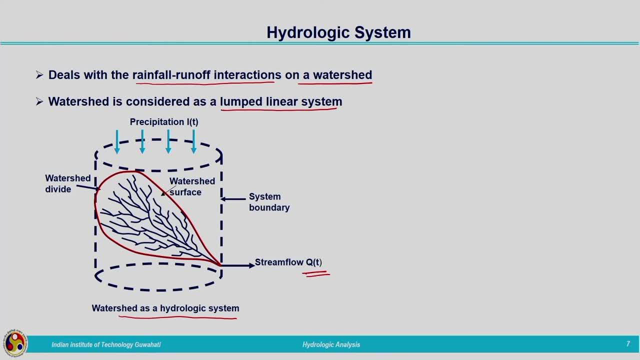 and here the example considered is a catchment- by means of a flow chart. we can explain it like this: rainfall is acted on the catchment, catchment is idealized as a lempt linear system and we are getting the runoff at the outlet which is represented by the hydrograph. so rainfall hydrograph is shown over here and the output is: 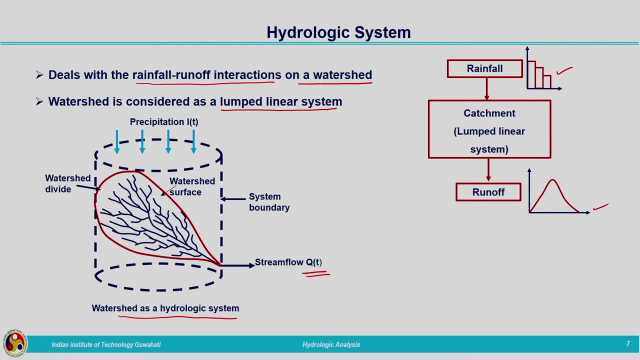 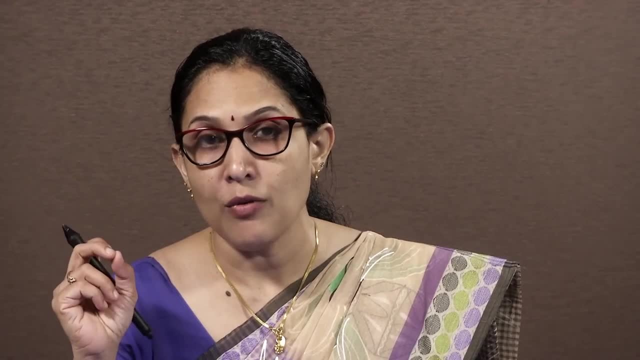 hydrograph- storm hydrograph- that we have already discussed in the previous module. the temporal distribution of flow at the outlet of the catchment can be schematically represented by means of a storm hydrograph. so whenever we are experiencing a rainfall, after deducting the abstractions or initial abstractions, 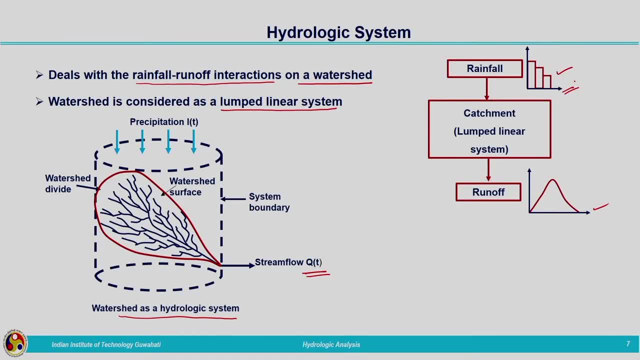 from the rainfall we will be getting the excess rainfall hydrograph. that is considered as the input to the hydrologic system and it is getting translated to direct runoff at the outlet. so that is represented by this direct runoff hydrograph. so we have seen storm hydrograph and from the storm 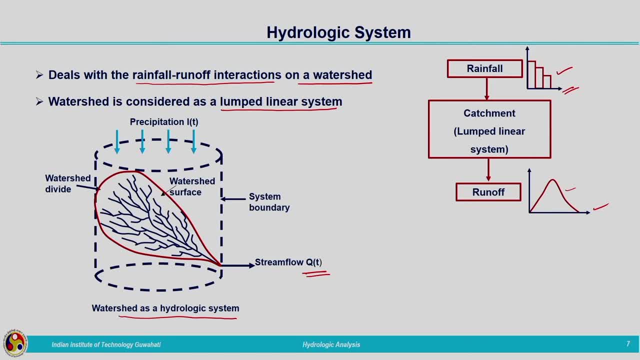 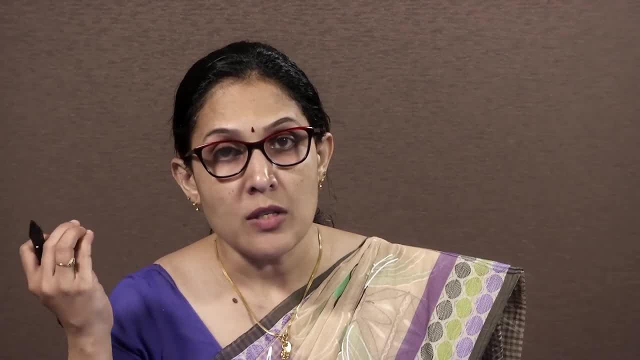 hydrograph based on the current flow of the hydrograph. the current flow of the hydrograph is base flow is separated by means of different techniques. after that, what is getting that is the direct runoff hydrograph, so excess rainfall is translated into direct runoff hydrograph. that is. 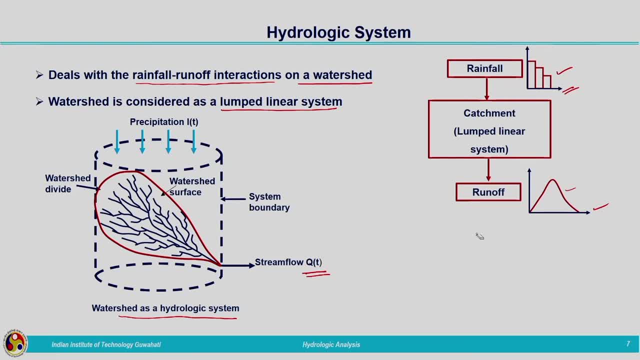 what is explained by means of this flow chart. so this is the conceptual model of rainfall runoff process, that is, it transforms rainfall excess to direct surface runoff, and one example for this is linear reservoir, in which storage is directly proportional to outflow. linear reservoir is an example for a 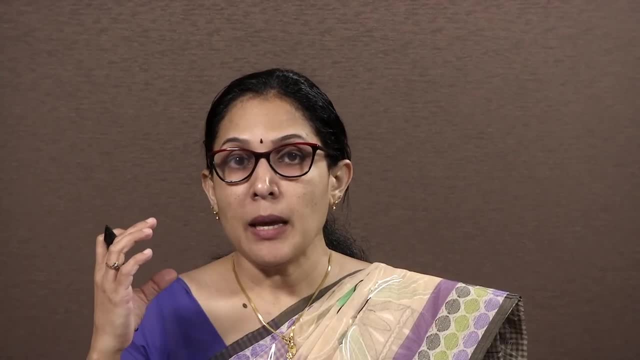 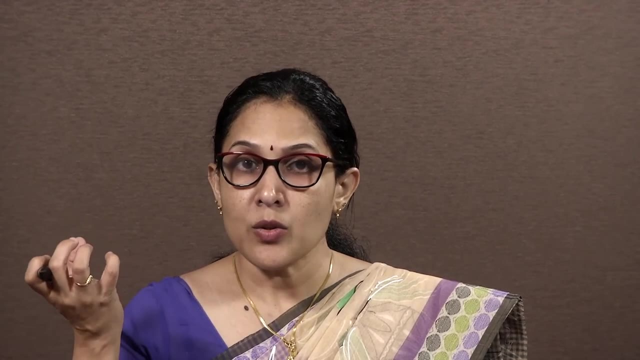 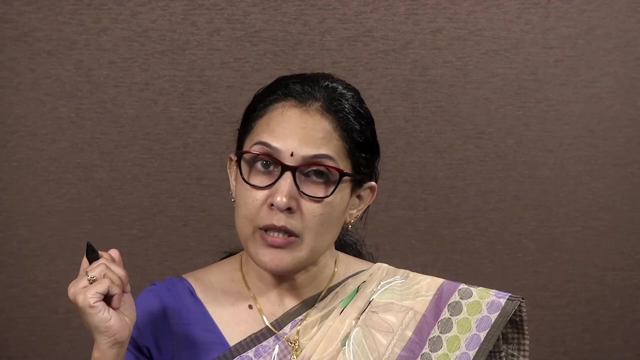 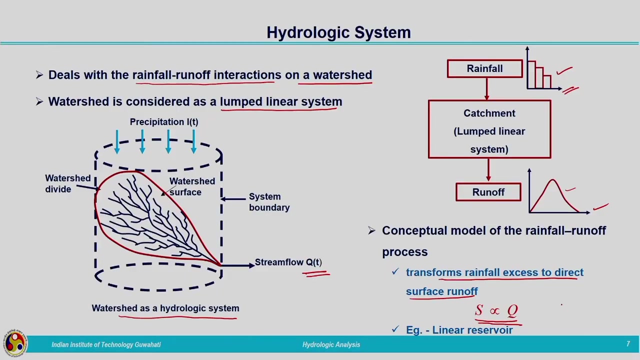 lemmed linear system, so catchment can be approximated by means of a linear reservoir. in this the assumption is that whatever storage is taking place within the catchment or the linear reservoir is directly proportional to outflow, or this proportionality constant can be removed and it can be written as s is equal to. 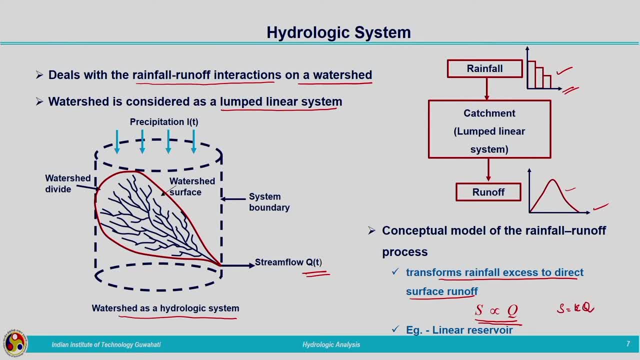 k, q. this k is representing the storage coefficient of the reservoir. so this way we can conceptually explain a hydrologic system, that is, the rainfall runoff process which is taking place in a catchment, can be conceptually explained by means of this figure and by means of a flow chart we can explain. 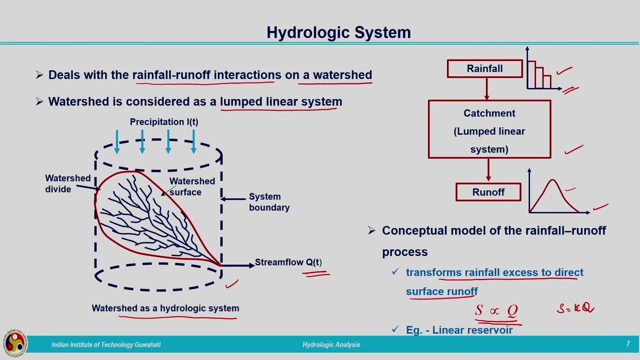 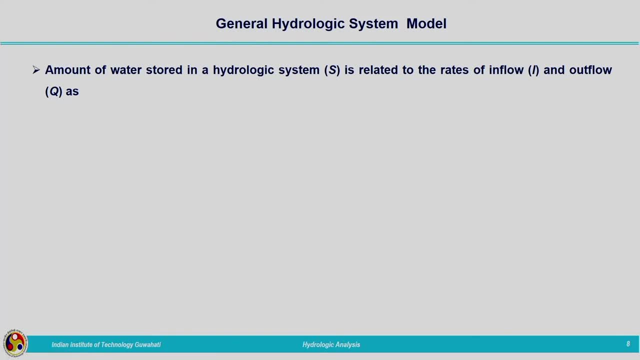 as explained with the of the flow chart on the right hand side. now let us move on to general hydrologic system model. so before going to the concepts which we are going to cover in this module, we need to have understanding about general hydrologic model. the amount of water stored in a hydrologic system. 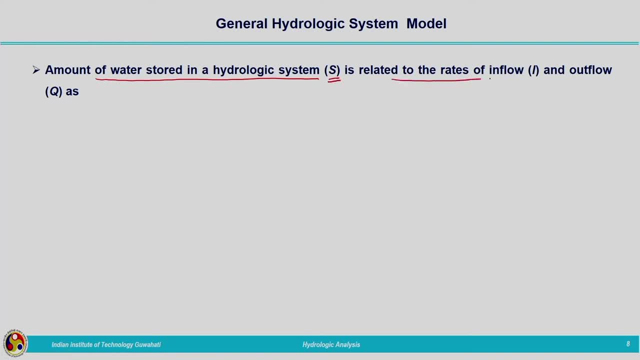 represented by capital s is related to the rates of inflow i and outflow q. that we know is whenever stream is in, flow is divided into, estabilised into causa, and outflow is the wrinkles of the cell function. and then how to find out thisUNF's charge order. 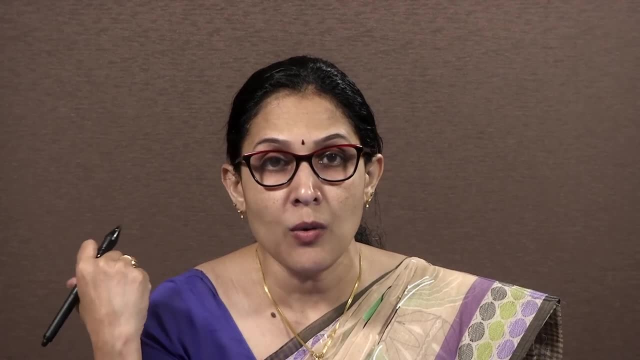 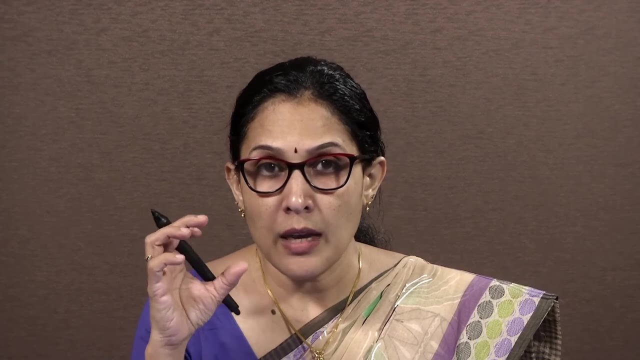 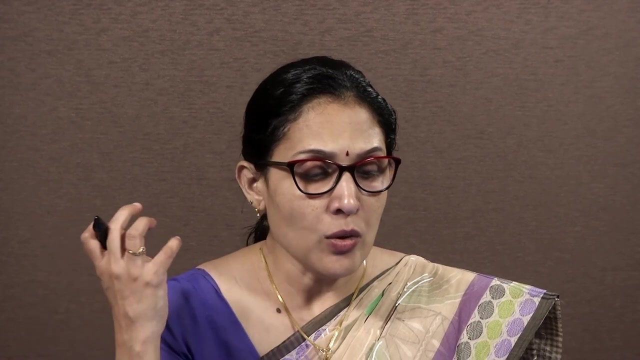 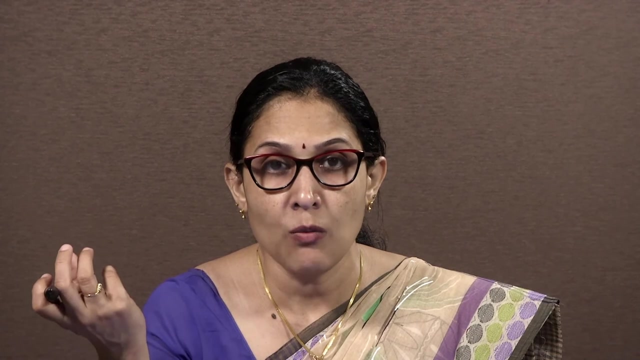 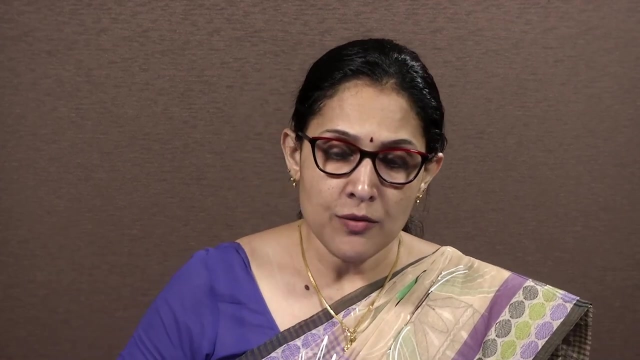 in which case the flow is going to depend on the rate of deflection of that flow. for example, it may be a watershed lake or any water body. it can be expressed in terms of inflow and outflow. so in the case of general hydrologic system model, the change in storage. 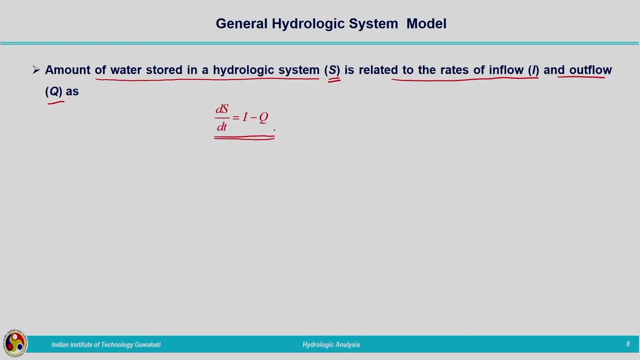 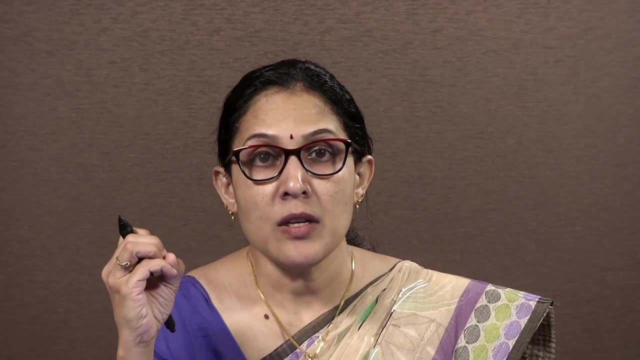 ds by dt is represented as the difference between inflow and outflow, i minus q. whatever amount of rainfall is occurring in a catchment, minus the outflow q. that is the abstractions. so those abstractions are represented by means of the change in storage. that is when we are 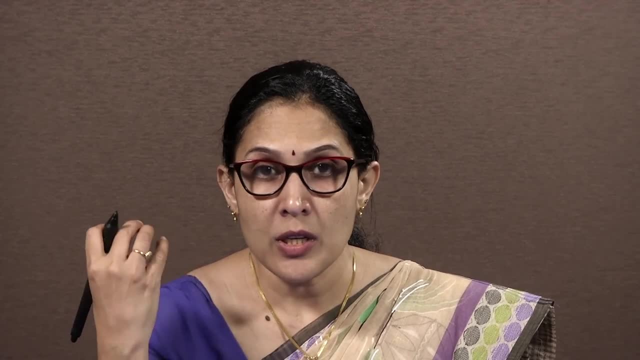 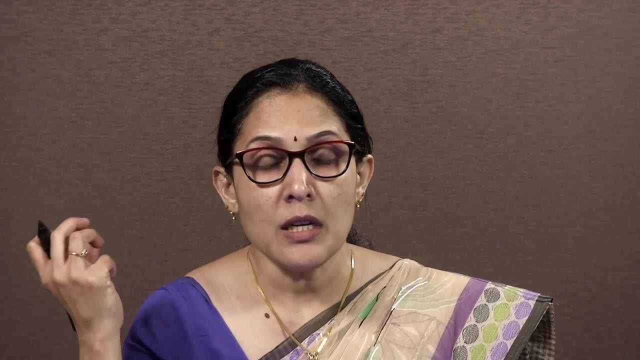 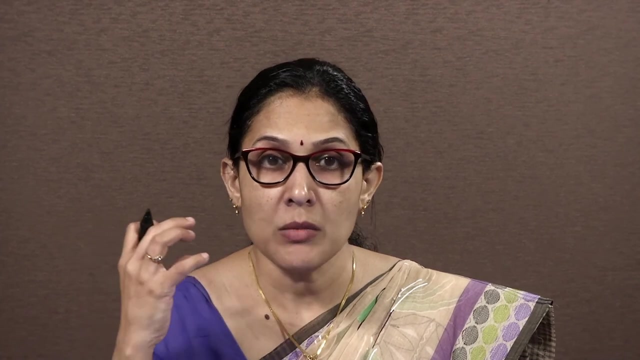 experiencing a rainfall after certain storage components are satisfied, we are experiencing the runoff at the outlet point. so whatever is experienced as runoff at the outlet point is okay by subtracting the abstractions from the inflow. So that is what is expressed here mathematically. 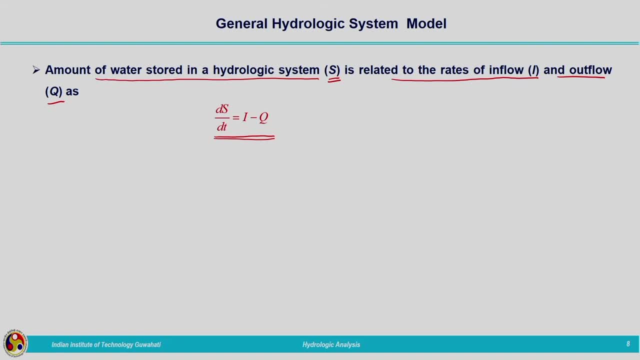 by means of this equation, that is, change in storage ds by dt is the difference between inflow and outflow. Let this equation be equation number one. Now, the amount of water stored at any time can be expressed by a storage function, So we need to express the storage which is taking. 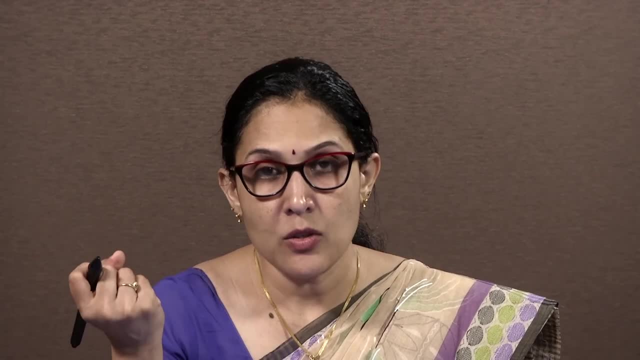 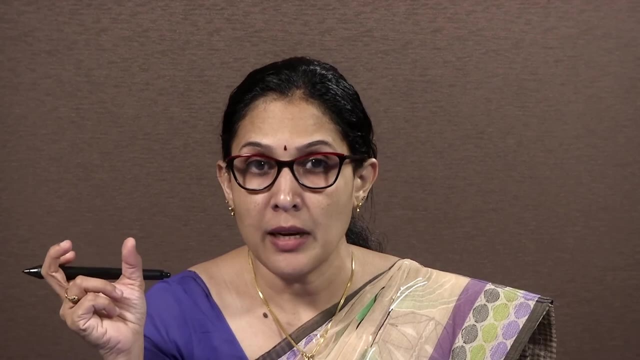 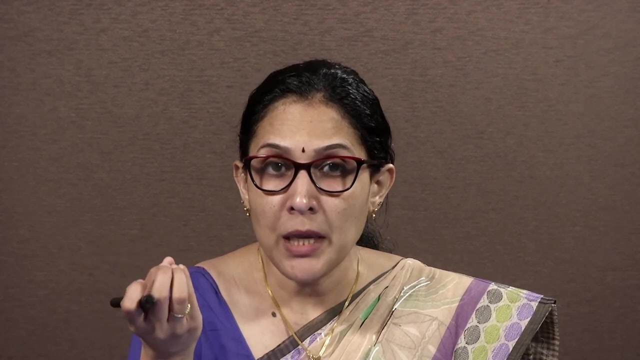 place in a catchment has to be expressed by means of a mathematical function. This, depending on the type of function which we are utilizing for representing the storage, our model will be accurate. If you are simply making use of a linear equation, y is equal to mx plus c. 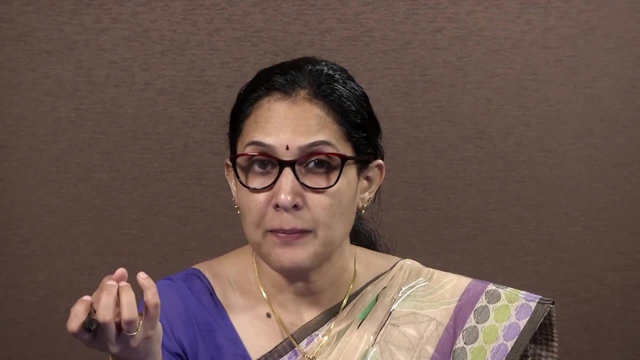 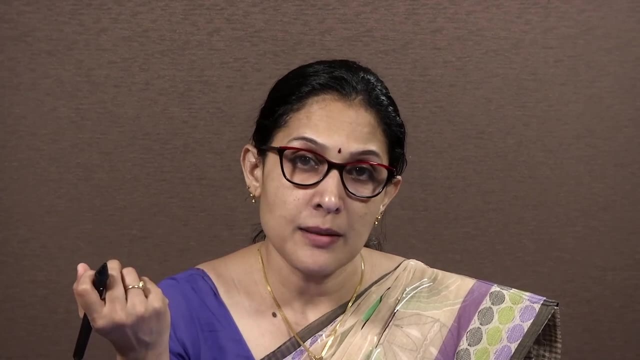 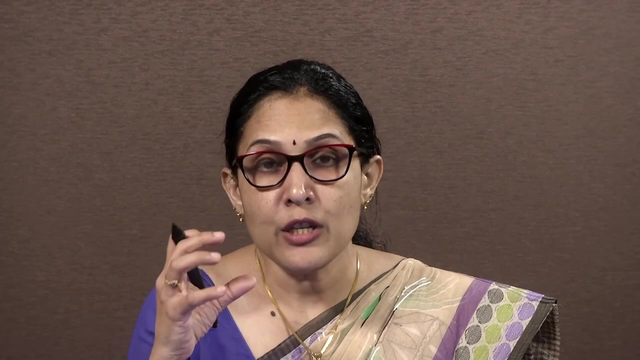 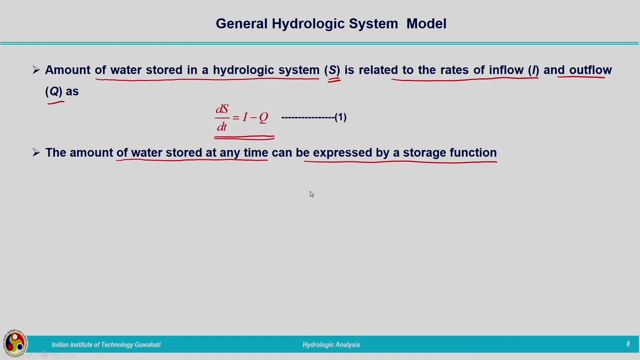 and your catchment is not behaving like a linear system, So in that case that model will be giving you certain output. That may not be the accurate result, So the research behind this is lying in the identification of the function which represents the storage accurately, So the amount of water stored in the catchment at 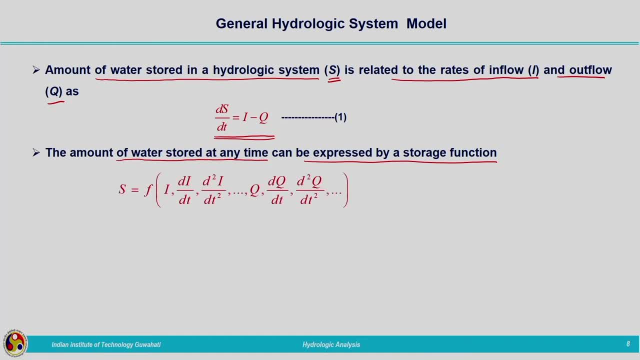 any time, can be expressed as a storage function that can be mathematically expressed by means of this equation. Let this equation be equation number two, That is, storage s. According to this example, stops are algunas as in infinite 2, less as in infinite constant. 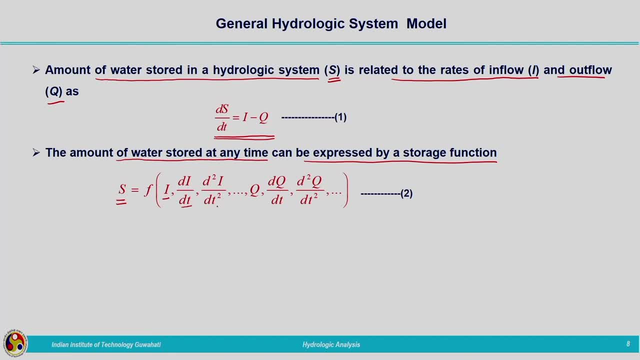 So from this signal to storage there is a function of inflow dh plus ket, of plus k to get oat root root k times k, Question 1. That TO and OT. Question 2 works against the frontal and clarify the true andterako relations of here is aコ. 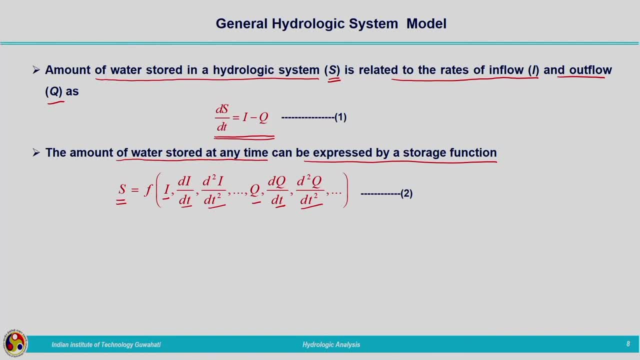 dp into dh s al sets. Let s dear that you have understood the definition of this system. Next, got to healthcare, which is healthy for you to stress the way you feel the body, things to be Why you are sick because you are not worried about the stress or you are into the. 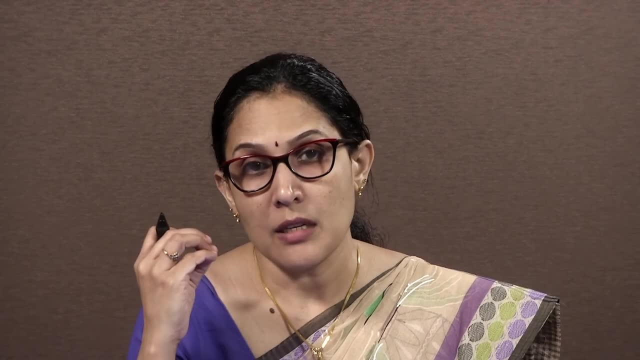 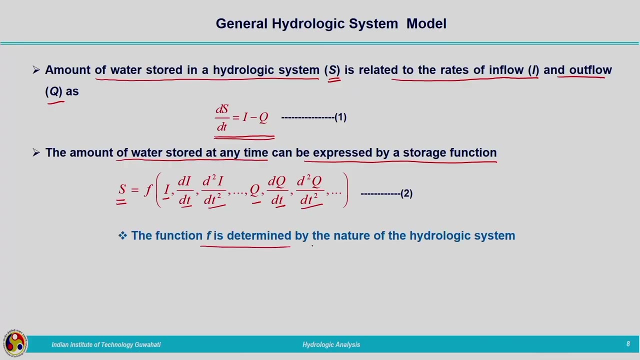 battery works. Let us take coke. Question 4. Question 5. Question 5. Question 5. Question 6. Question 7. Question 7. Question 13. Question 14. Question 14. Question 12. Question 11. Question 13. Question 12. flow, outflow and the derivatives. The function f is determined by the nature of the hydrologic. 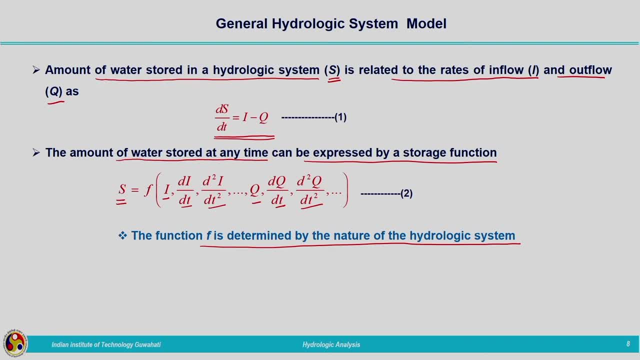 system. That is what I told you. This particular function depends on the type of the hydrologic system which we are considered. This storage function can be represented by means of a simple equation, or we can incorporate all the complexities involved with the catchment by making use of a. 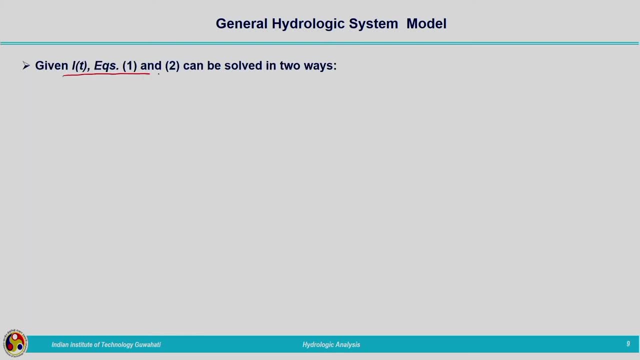 complex function. Now, given I t, equation 1 and 2 can be solved in two different ways. One is by means of analytical method and second is by means of numerical method. That is an approximate method. This is for your understanding only. I am explaining here. If we are having 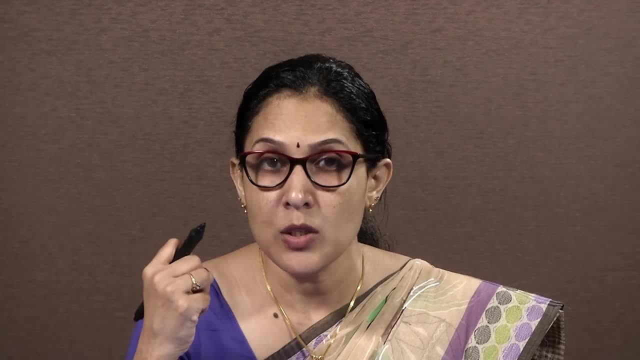 certain equations representing a system. how can it be solved? Because here our intention is to find out the stream flow rate of the hydrologic system. So we are going to find out the stream flow rate of the hydrologic system. So we are going to find out the stream flow rate of the. 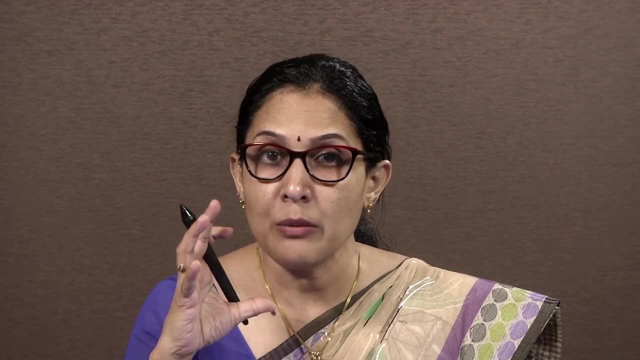 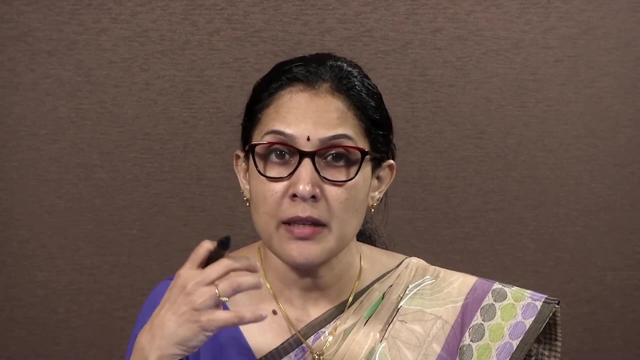 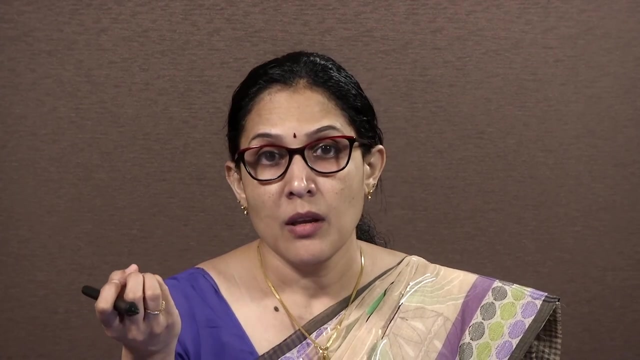 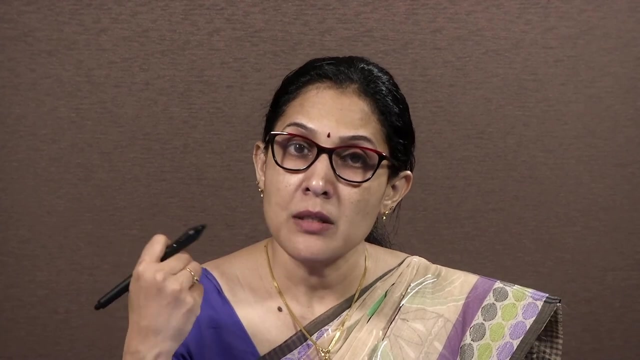 outlet. So for that we need to solve the equations representing the catchment mathematically. So we are having the mathematical function representing the storage component. So we need to make use of certain mathematical techniques to solve this equation. So how can these equations be solved? Either we can make use of analytical techniques or by 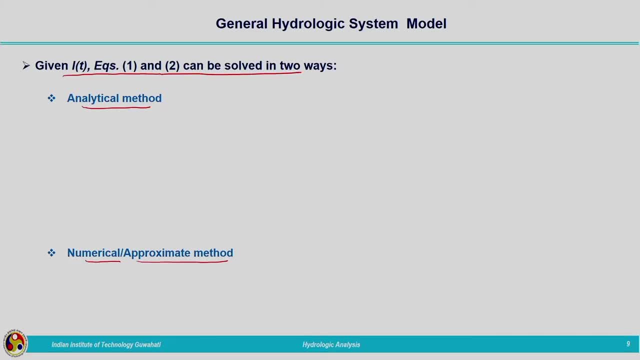 means of numerical techniques, So analytical method, what we are doing. this is our equation representing a storage function. We can find out ds by dt using the equation 2.. That is, ds by dt is equal to I minus q difference between inflow and outflow. So from this equation we will 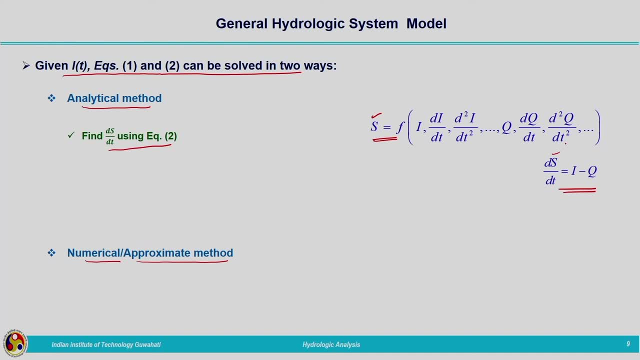 be finding out ds by dt. We will be substituting here over in this particular equation. So what we are making use here, method of substitution, So substituting into equation 1 to get the governing difference. So we are making use of the method of substitution, So substituting into equation 1 to get the governing difference. 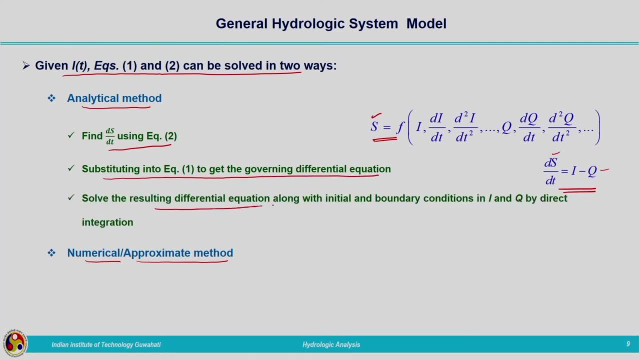 Now the resulting differential equation can be solved by making use of the initial and boundary conditions in input I and output q, by direct integration. That is, we are having a differential equation in terms of ds by dt, So that can be solved by integrating that. For integrating that: 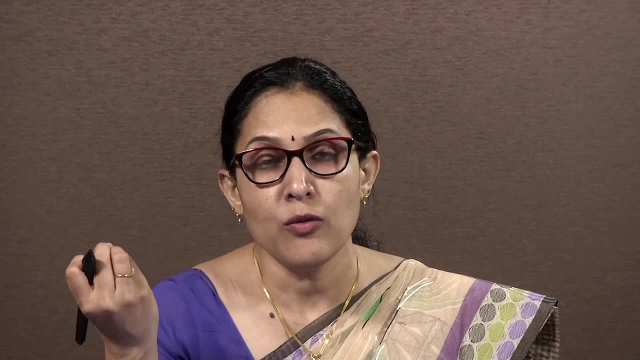 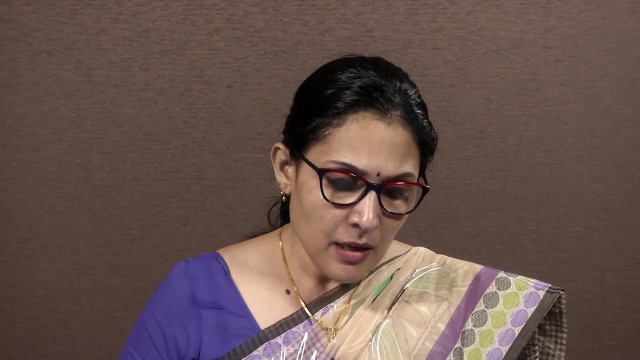 we need to have certain understanding about the inflow and outflow, because storage is a function of inflow and outflow. That is what is done in the case of analytical method, In the case of numerical method or approximate method. a finite difference. approximation of equation 1 and 2. 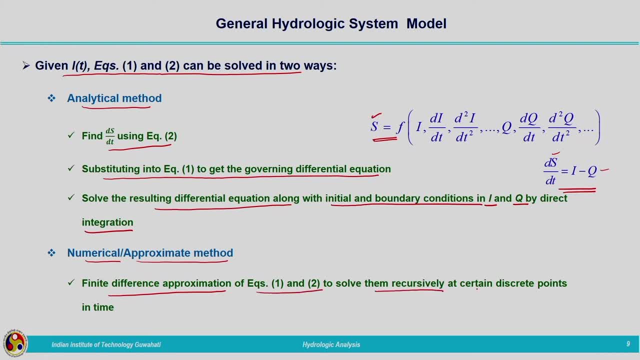 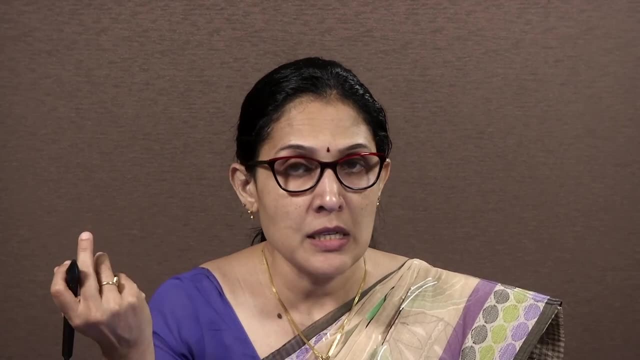 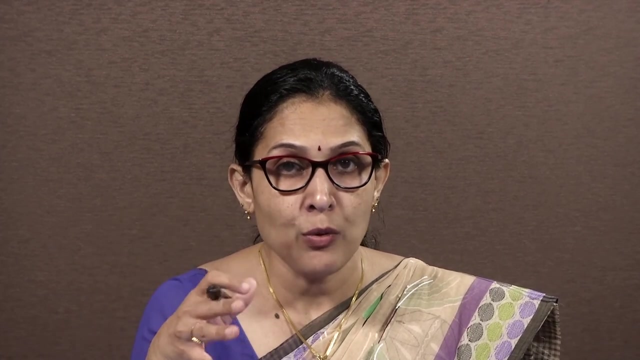 will be utilized to solve them recursively at different discrete points in time. So these finite difference method or different numerical techniques you will be studying under another course on numerical methods, numerical applications in engineering. So that is beyond the scope of this scope. But for a basic understanding I have put this: 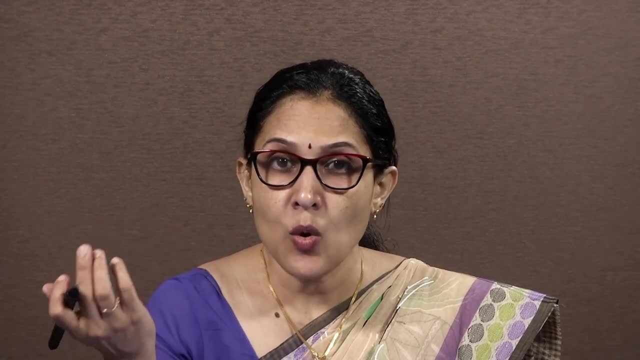 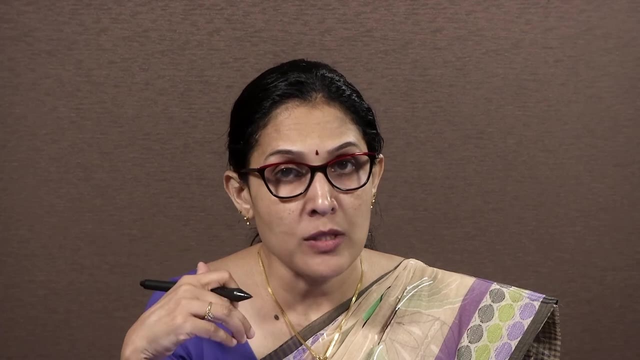 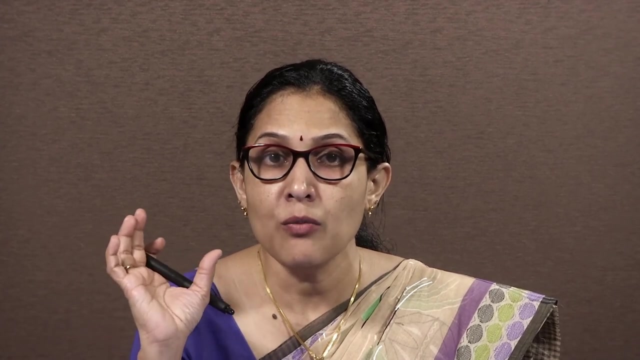 slide over here how this equations can be solved mathematically. That is, either by means of accurate solution or by means of approximate solution. Getting accurate solution always will be difficult, Depending on the complexity involved with the equation. solving analytically will not. 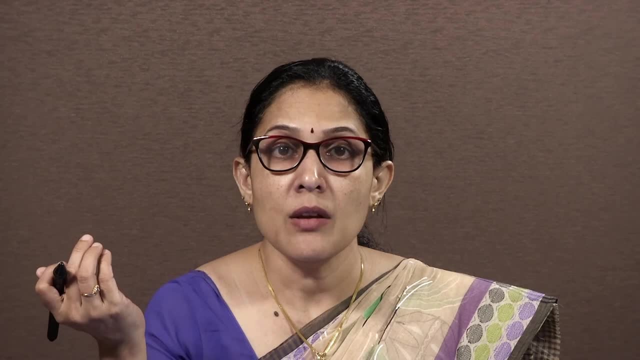 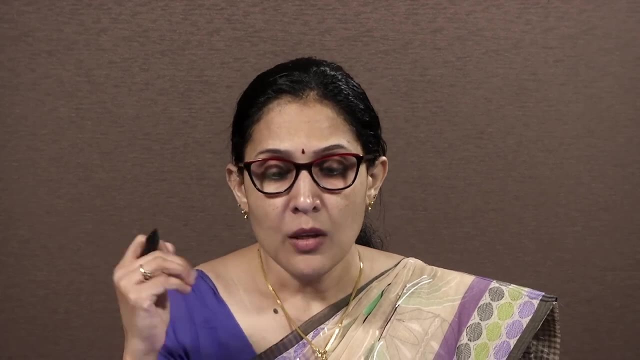 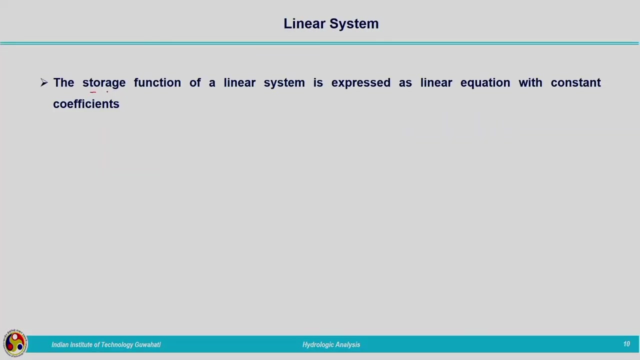 be possible. So in such cases, without compromising on the accuracy or of the results, we can make use of numerical techniques. So these are the two ways in which we can solve these equations. Let us move on to a linear system, That is, the storage function of a linear system is: 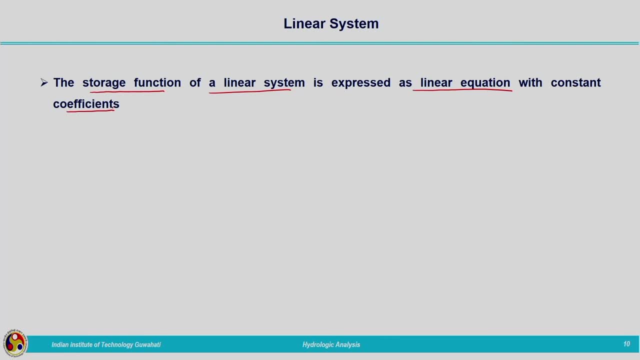 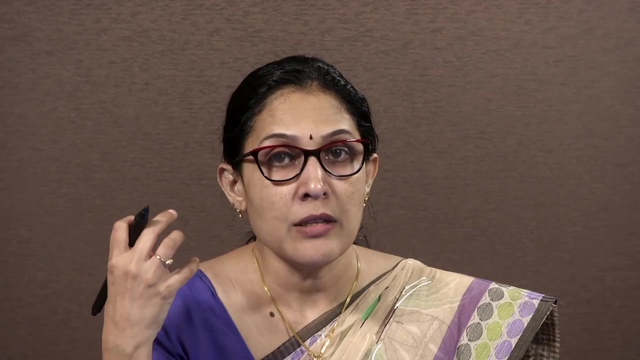 expressed as a linear equation with constant coefficients. The system can be linear and non-linear, Depending on the complexities involved with the system. it can be non-linear or if the system processes which are taking place in the system are simple and if it can be conceptualized by means of a linear equation, it can be expressed as a linear. 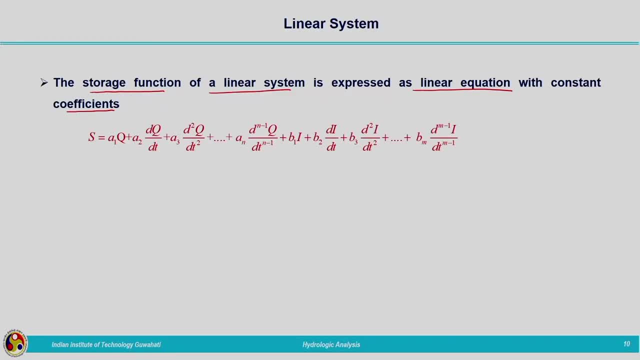 system. Here we are going to look into a linear system in which the storage is expressed by means of a function given by this equation. S is a function of outflow Q dQ by dt d square, Q by dt square. This is the function of outflow Q dq by dt d square, Q by dt square, d square Q by dt square. 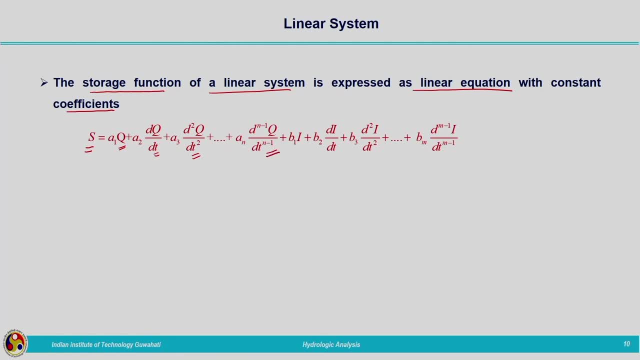 to nth derivative we have considered In the similar way. it is a function of inflow, i derivatives of i, di by gt d square, i by dt square up to m minus 1 derivative. So storage is assumed as a function of inflow and outflow and their derivatives. Let this equation be equation number. 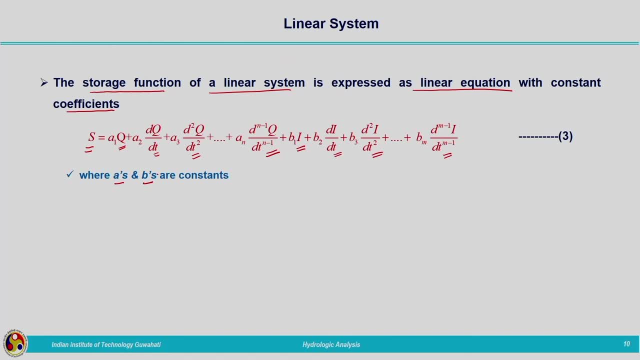 3, and here a's and b's are constants. a's are coefficients of outflow q and their derivatives, and b's are coefficients of inflow i and their derivatives. These coefficients are constant coefficients which are time invariant. With respect to time, there is no change taking. 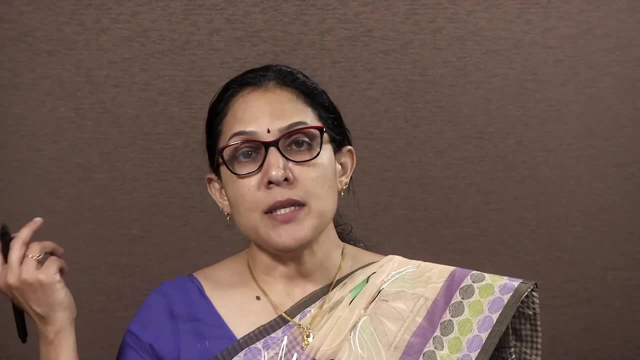 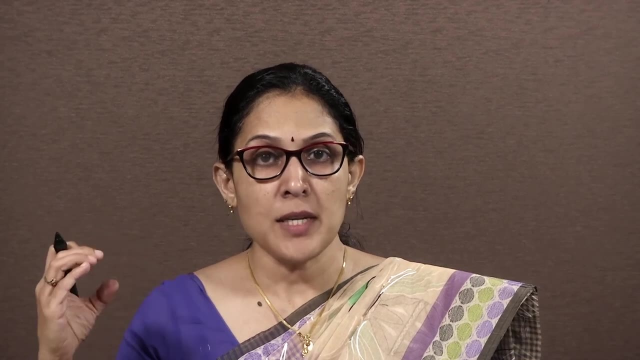 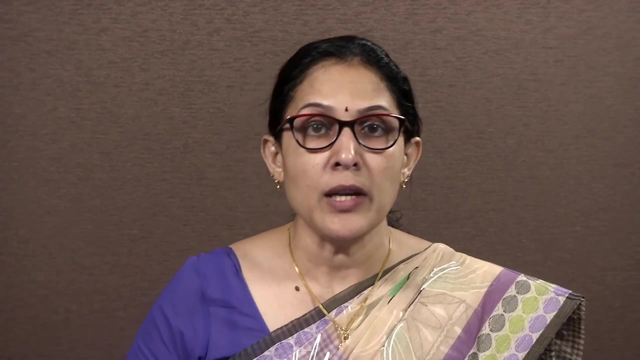 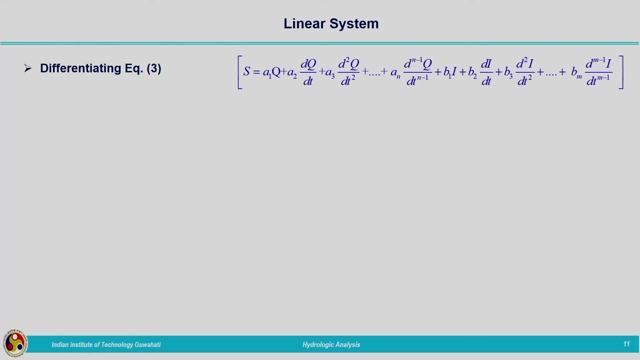 place with these coefficients. Now, next step is that to differentiate that particular equation representing storage, That is, s is expressed as a function of inflow, outflow and their derivatives. Now we need to differentiate that particular equation. We need to get the value corresponding to ds by dt. This is our equation representing s. 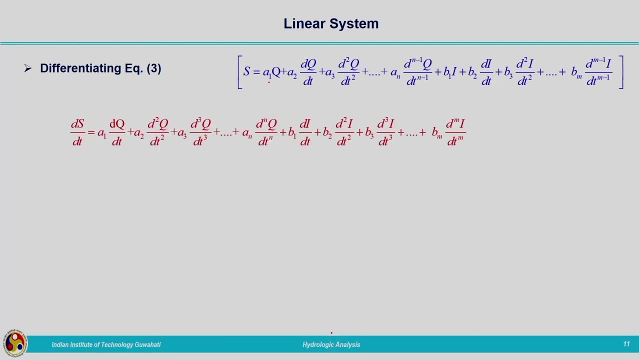 and ds by dt. If you are differentiating this a1 dq by dt, a2 d, square q by dt, square a3 d3 q by dt cube, that way it goes up to last term corresponding to q will be a n dn q by dt. 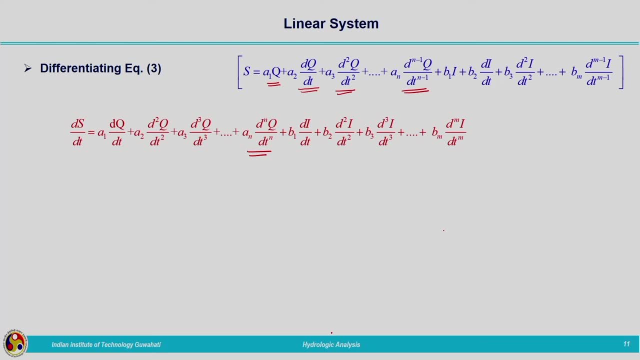 n. Now coming to inflow terms: b1 di by dt, that is given over here. b1 di by dt. b2 d square- i by dt, and b3 d cube- i by dt cube, and last term will be dm, dm i by dt, to the power of m. So we have 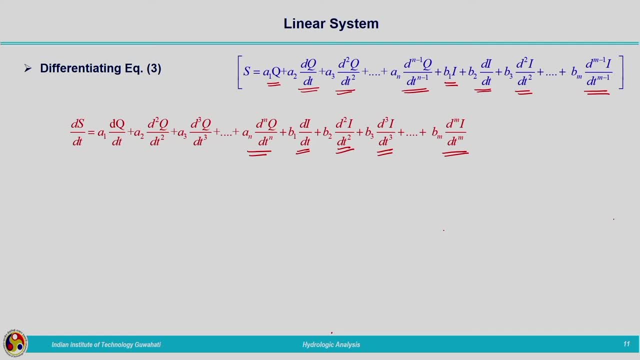 differentiated with respect to time and that equation is written over here. And we know ds by dt is equal to i minus q. So here in this equation for ds by dt, we will substitute this expression, So that we will be substituting and we can write i minus q. 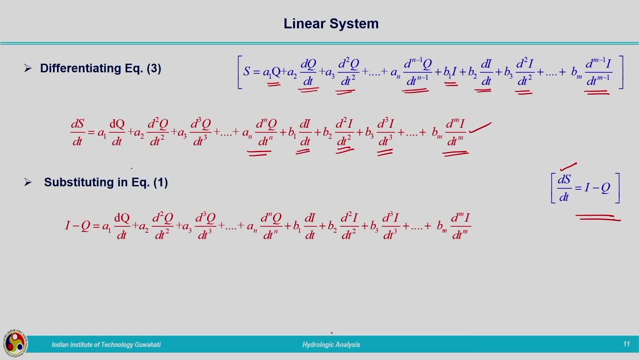 is given by the right hand side of this equation, right hand side of this ds by dt, So that we have substituted over here i minus q is here on the left hand side, and we are having i and q terms on the right hand sides also. So now we will do certain kind of rearrangement. 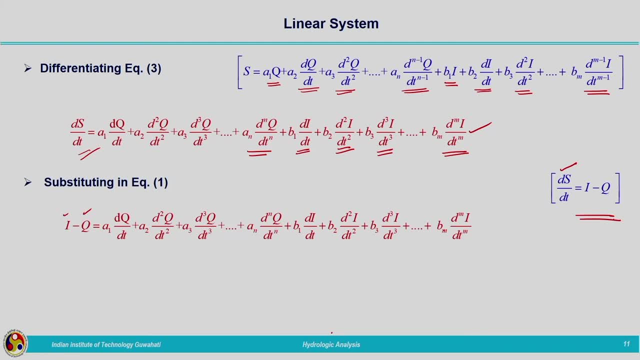 in such a way that all the i terms on one side and all the q terms on the other side. That way, if we are rearranging the equation, we have taken all the q terms to the left hand side and all the i terms to the right hand side. So you can get an equation: a, n, dn, q, dt, n plus a, n. 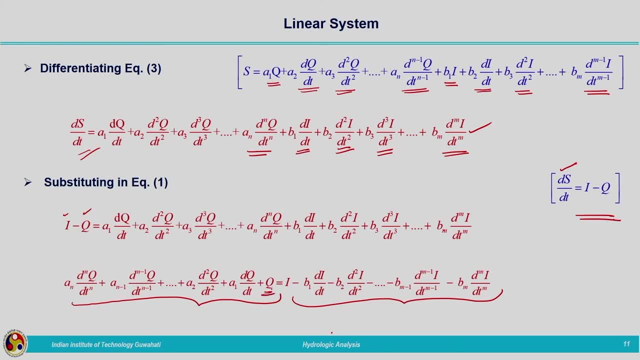 q by dt. n minus 1 up to q, And on the right hand side, i minus b1. di by dt up to minus bm. dmi by dtm. Let this equation be equation number 4.. This is the general hydrological system model. 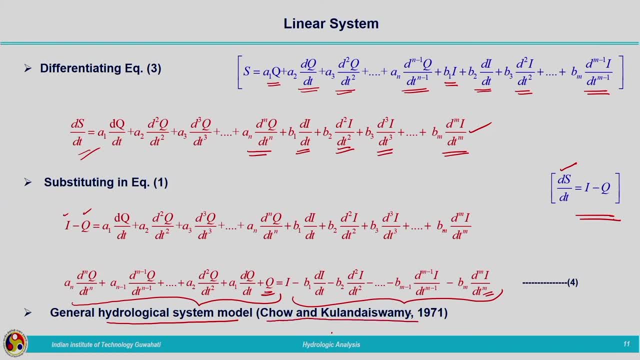 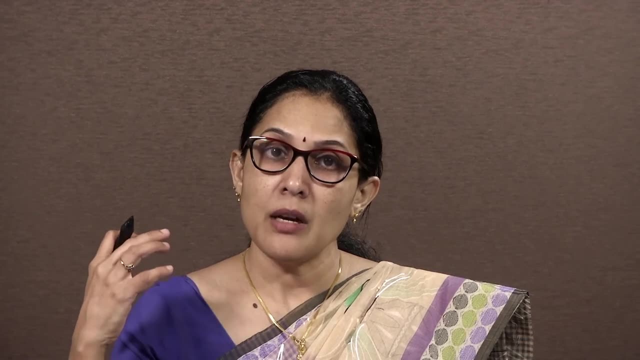 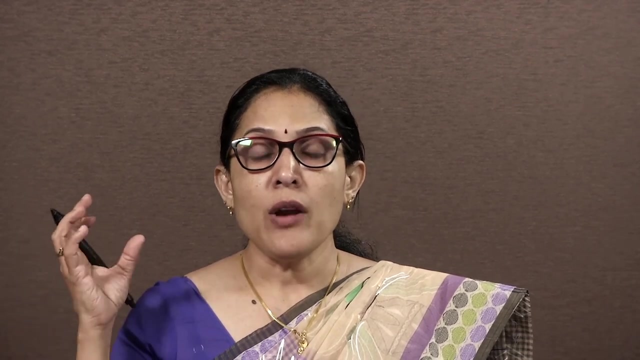 This has been proposed by Chauhan Kulenday Swami. So this is the general representation of a linear hydrologic system. In this, each component is expressed as a linear equation, which is a function of input and output: inflow i and outflow q and their derivatives. So what we have done: function is assumed as: 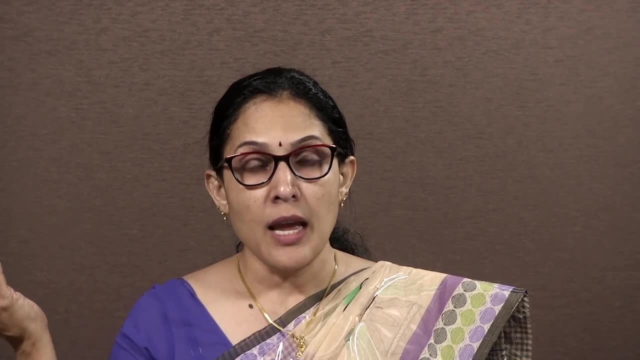 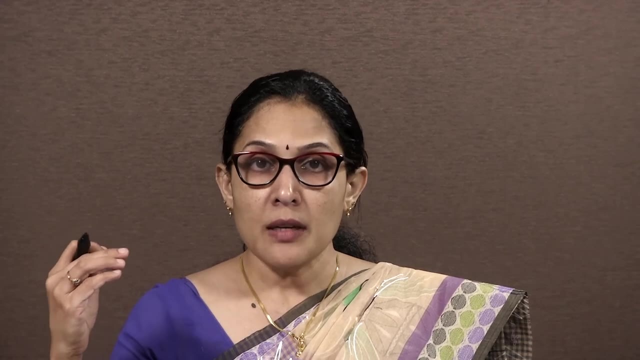 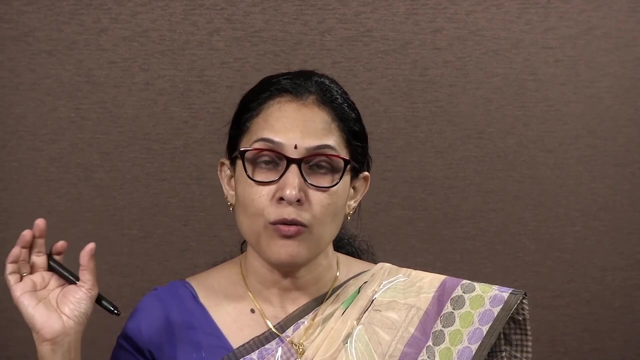 a linear function in i, q and their derivatives. And we know the general expression for rate of change of storage. That is represented by change in storage, that is, s by dt is nothing but the difference between inflow and outflow. Precipitation is occurring. 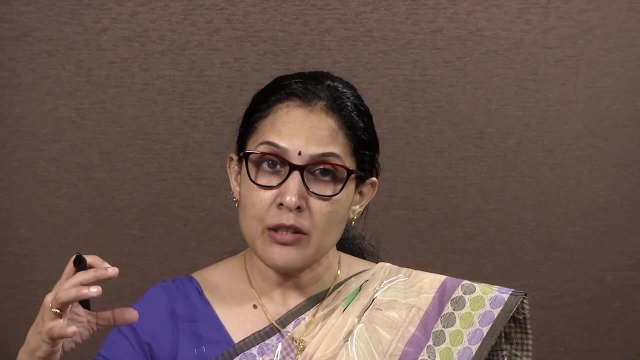 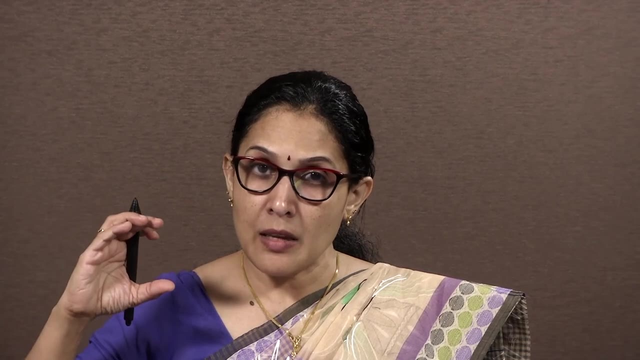 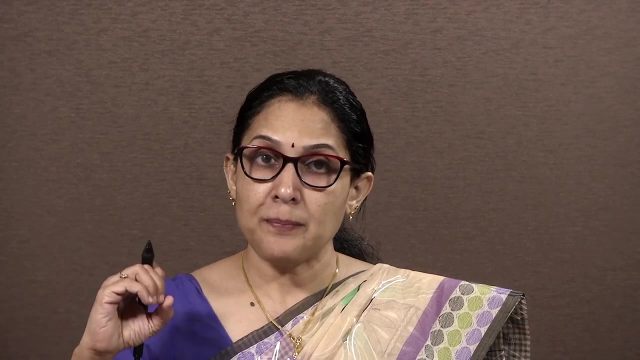 Out of that certain water is lost to satisfy different storage components. Remaining is coming as the outflow. So inflow minus outflow is assumed as the storage component. That storage is represented by means of a linear equation. That linear equation is a function of inflow. 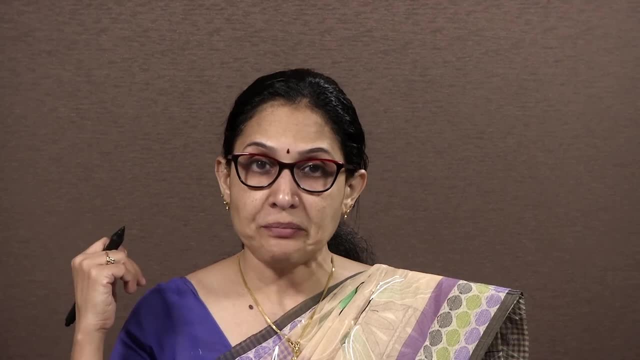 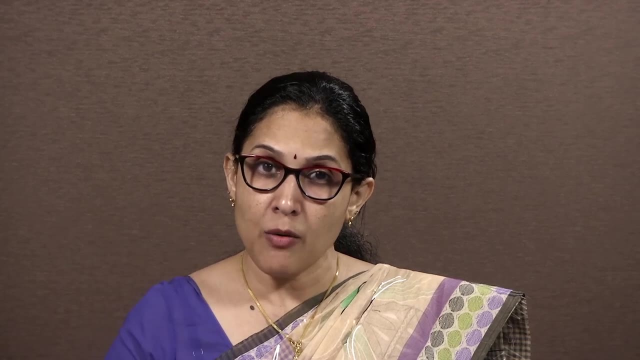 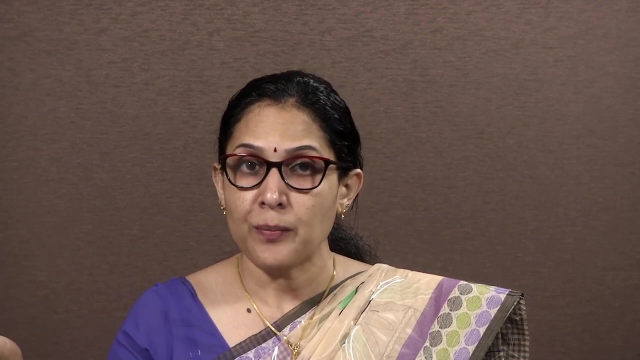 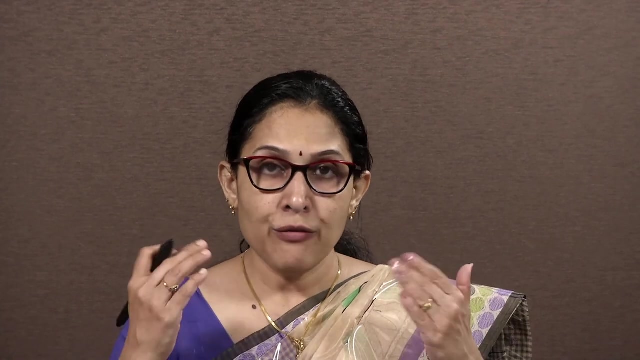 outflow and the derivatives, So all the terms we have considered. After that, what we have done, ds by dt expression found out That has been substituted in the equation: change in storage is equal to difference in inflow and outflow. After that we have found out a general hydrologic system model by differentiating and: 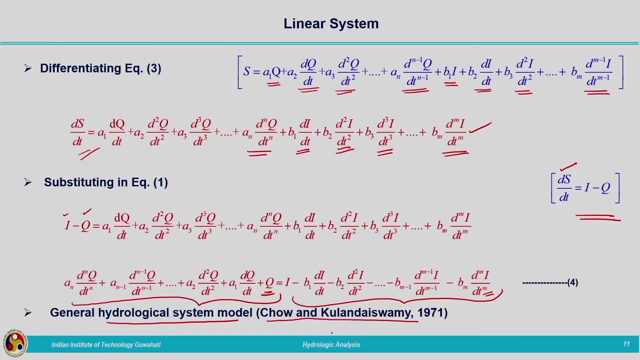 rearranging certain terms. So the equation 4 is representing the general system model. So we have found out a general system model by differentiating and rearranging certain terms. So the equation 4 is representing the general system model. So the 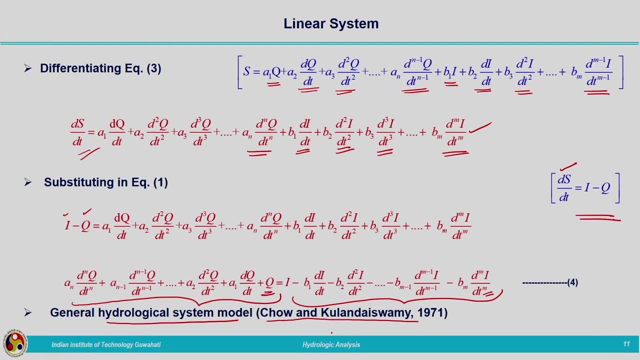 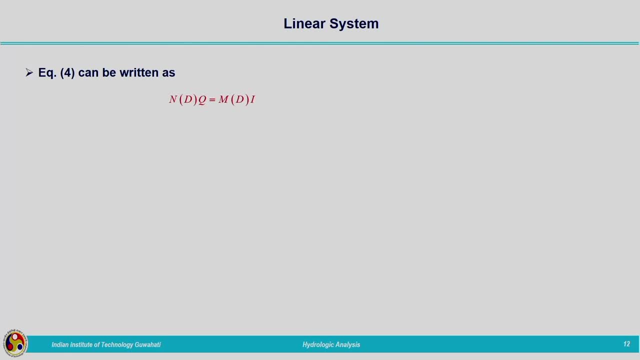 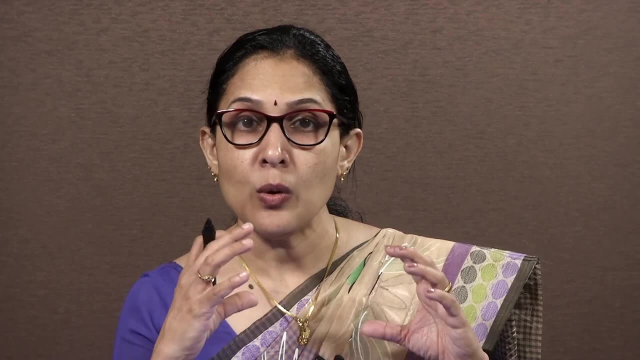 equation 4 is representing the general hydrological system model proposed by Chauvin Kulandeswami. Now that can be rewritten again. That is the entire term. carrying entire term together will be difficult, So we are making certain substitution in order to look at very 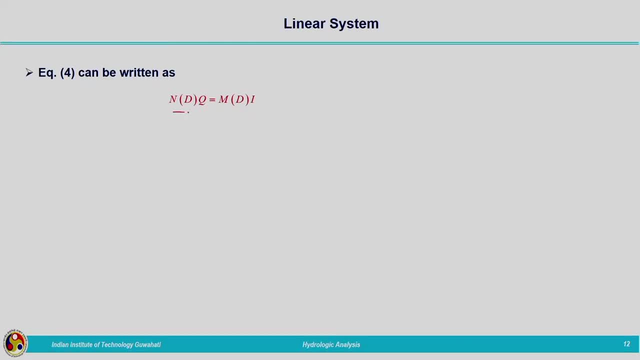 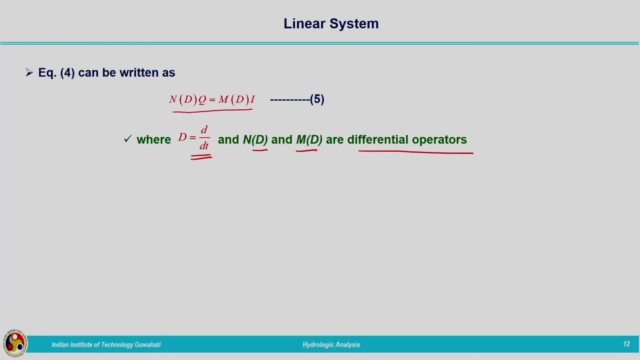 dt terms are the differential operators, So all the differential operators combined together: related to q, it is put under nd, and related to inflow i, it is put under md. And if you want to get the output, that is qt. qt can be written as md divided by nd, multiplied by it, So md by nd. 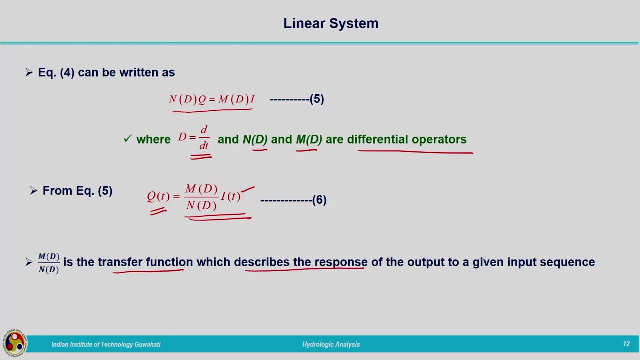 is the transfer function, which describes the response of the output to a given input sequence. You can look at the equation that is represented by equation 6.. I t is our input. For example, it is rainfall That rainfall is causing the runoff. Our intention is to find out the impact of this hydrologic variable. 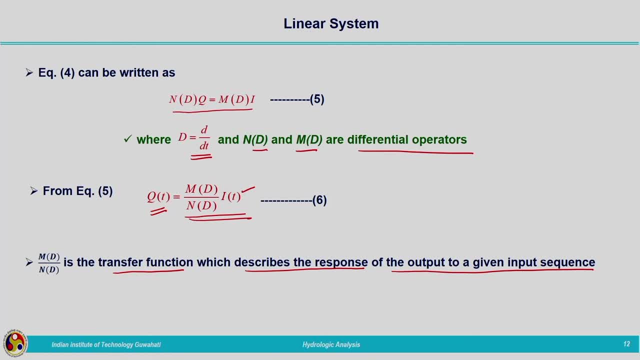 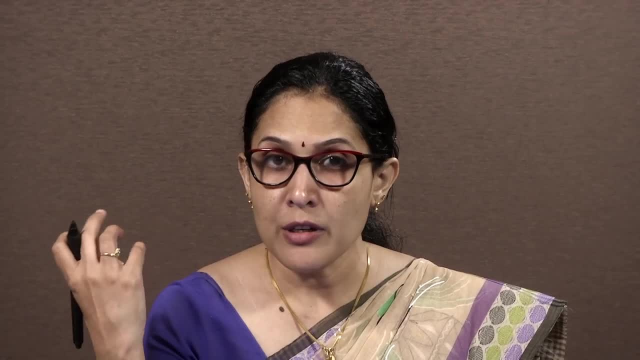 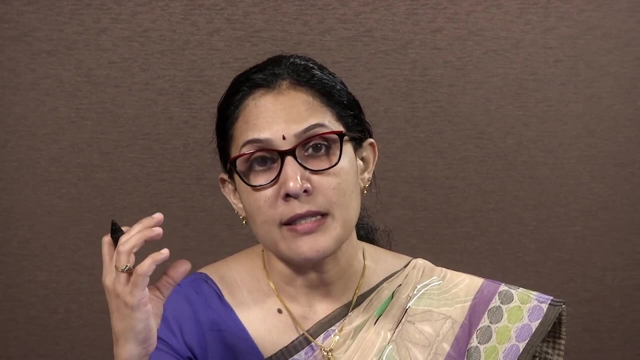 rainfall That is represented in terms of Q, t, in the form of outflow or in the form of stream flow. Calculating the stream flow as a function of inflow, we can make use of this equation. So for this, in the case of a general hydrologic system, the input is translated to output by means.